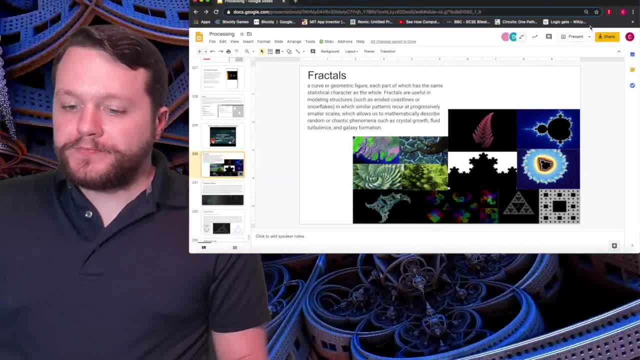 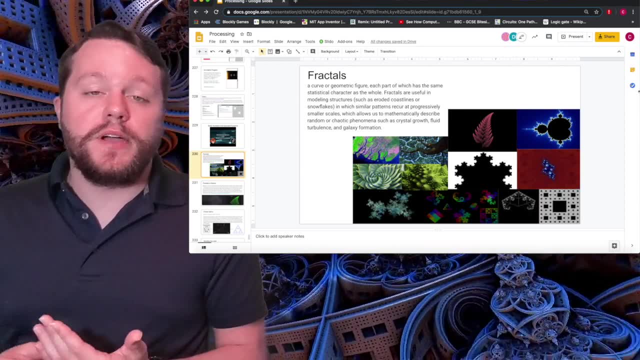 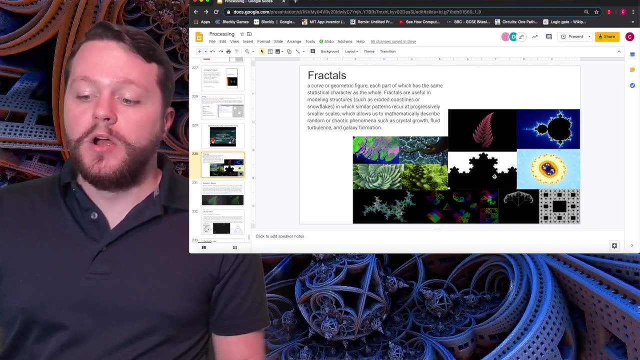 Let's take a look at the slides I have for you here. So a fractal is just a curve or geometric figure where each part has the same statistical character as the whole, meaning it's self-similar at different scales. So if we zoom in, like if we look at the Coke snowflake right here, we see the same. 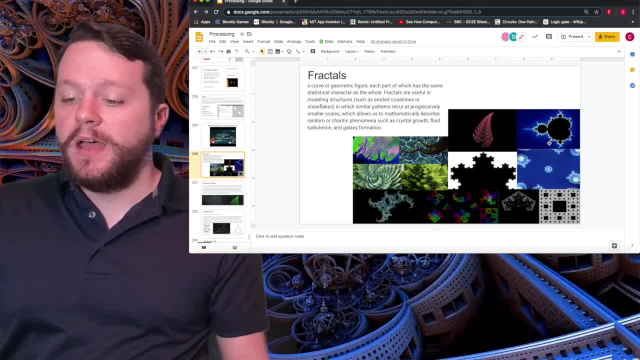 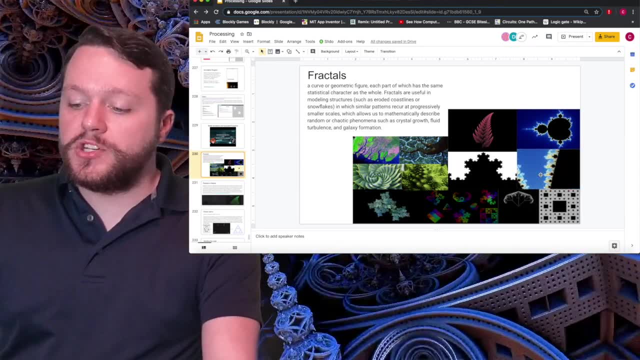 structure, No matter how much we zoom in, we'll continue to see this. Now, over here, this is a pretty famous fractal called the Mandelbrot set, And down below it we have a little gif showing us this self-similar nature. As we zoom in we can see a lot of different structure, but there's the. 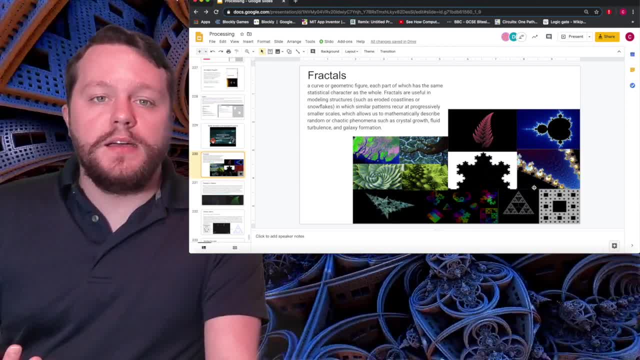 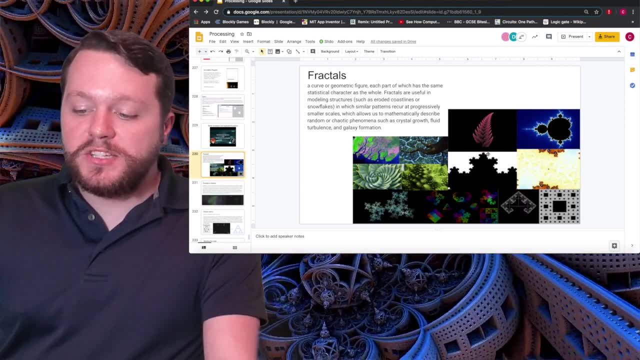 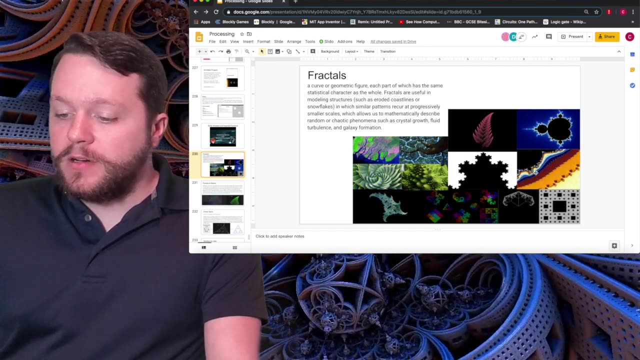 Mandelbrot set again. So we see the self-similarity at multiple scales. And, by the way, I love this fractal, Each fractal that you see here. you can infinitely zoom in and still find patterns. Here this fractal, this Mandelbrot set, was zoomed. Oh, there it is again. I don't know how many. 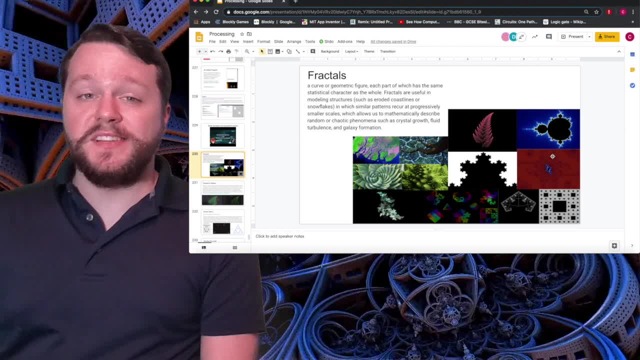 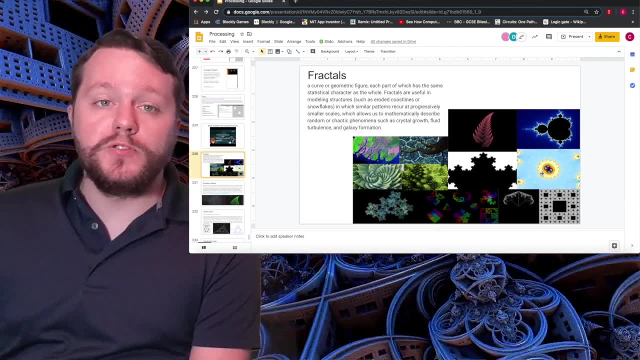 iterations they had to do to make that happen. It happened a ton, but that's awesome. The color just comes from. Now this is a little bit mathy, but so a point: how quickly it goes to infinity is given a color. 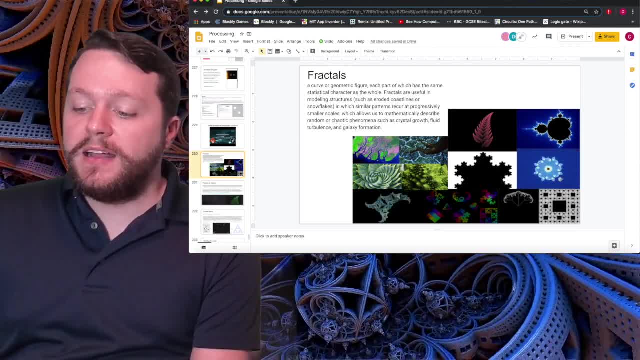 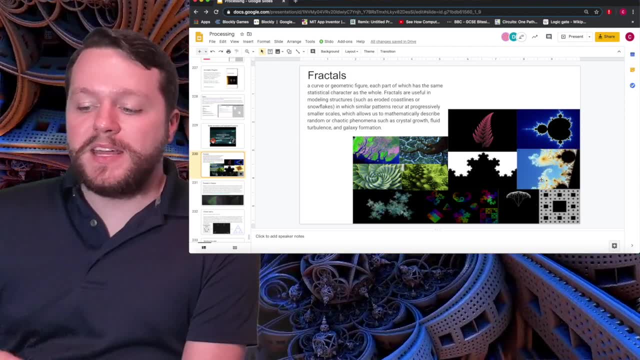 So that's why this is so colorful. Really this is just black and white. They added the color to show how quickly points go off to infinity, to just add a little bit more complexity and make it a bit interesting. And you can see all kinds of fractals here. We have plenty of fractals in nature, Nature. 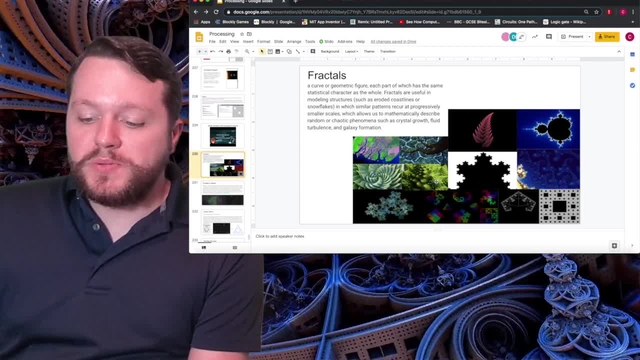 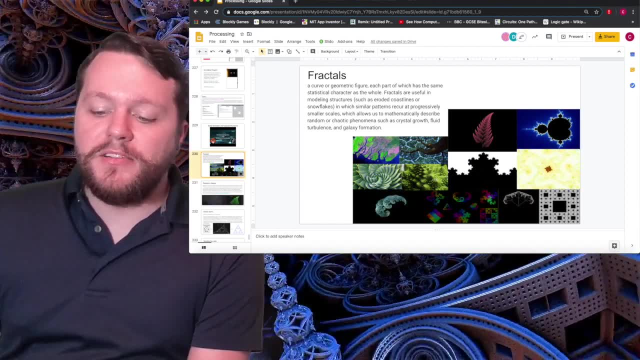 is fractal, So here this is just broccoli, but you can see that little spiral pattern in each of them. I don't even know what you call those, I'll just call them green things. In this we have a little spiraling plant. We can see fractal patterns inside of trees, the way that they branch off. 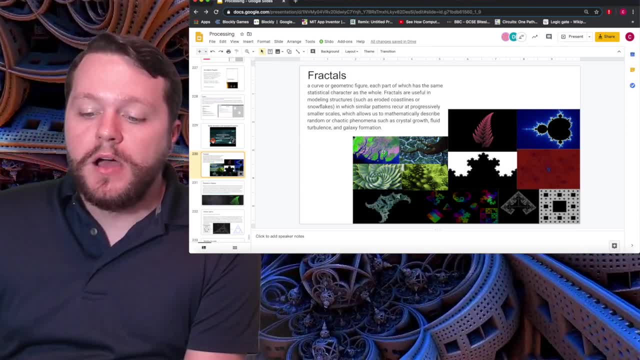 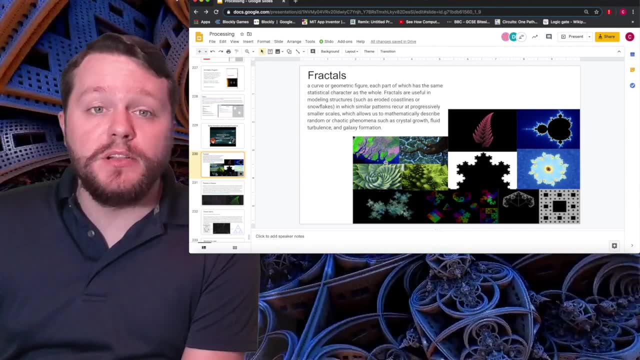 and in rivers and lakes. So if I were to zoom in on this coastline, we would see more and more of that kind of wiggly pattern for those rivers right, It's self-similar at multiple scales. I can zoom in and see more and more self-similarity. So let me continue reading this part. 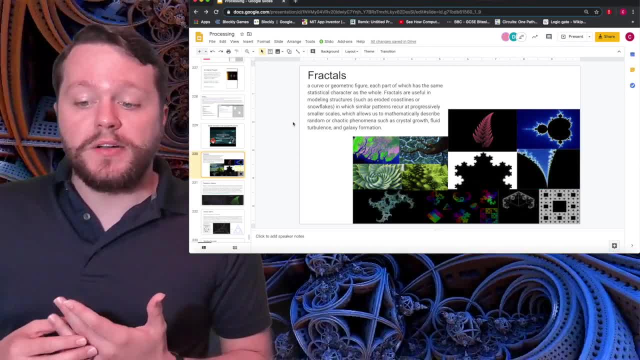 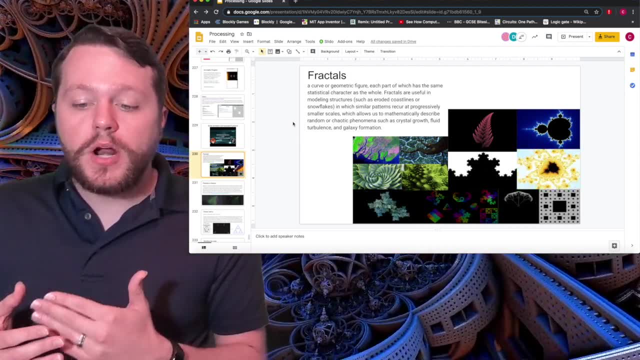 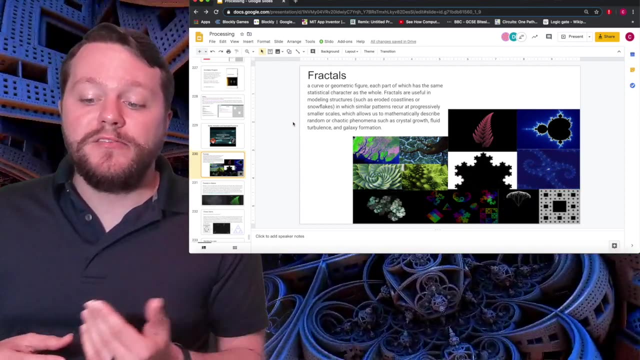 useful in modeling structures such as eroded coastlines, snowflakes, lightning, you know whatever, And these patterns recur at progressively smaller scales. like I was just saying, This allows mathematicians, computer scientists, to describe random chaotic phenomena such as: 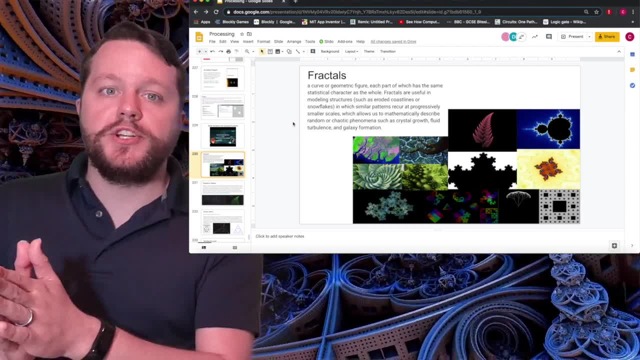 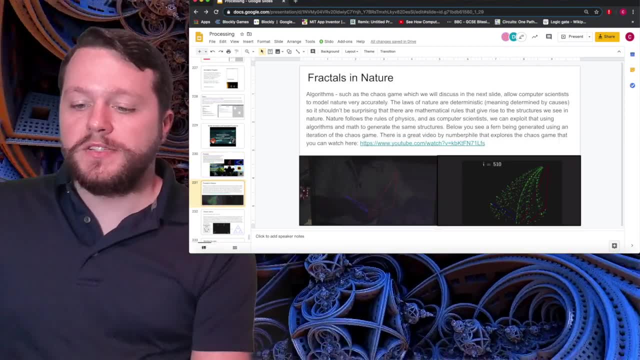 crystal growth, fluid turbulence and dynamics, galaxy formation, And using this math, we can then simulate it to create things digitally. So let's keep moving. So here we can see a little bit of an example of that. So this is a fern that's being generated by the 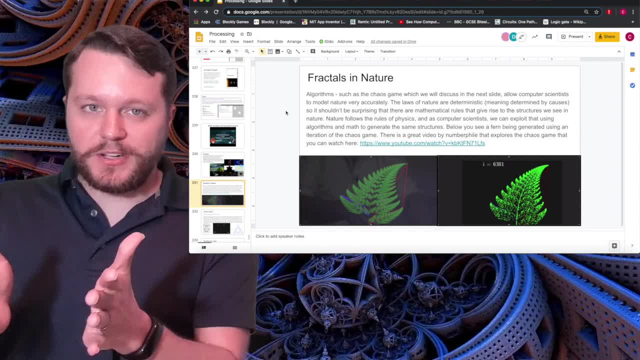 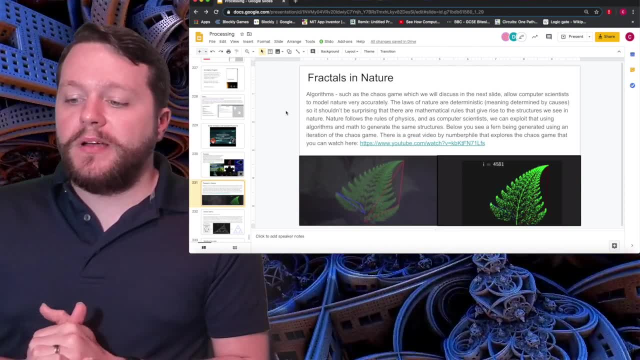 chaos game, which we're going to talk about in the next slide. So let me go into what exactly is happening here. Algorithms such as the chaos game- the thing that we're doing today- allow computer scientists to model nature very accurately. The laws of nature are deterministic, meaning they're 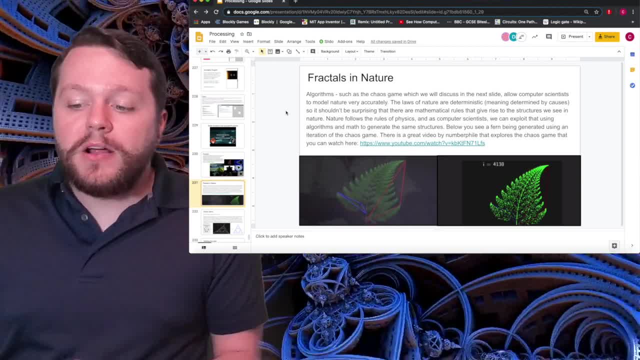 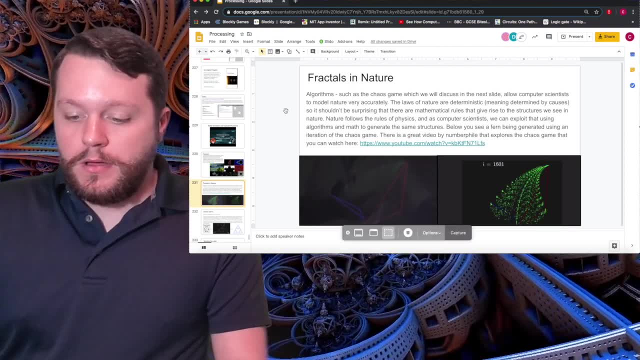 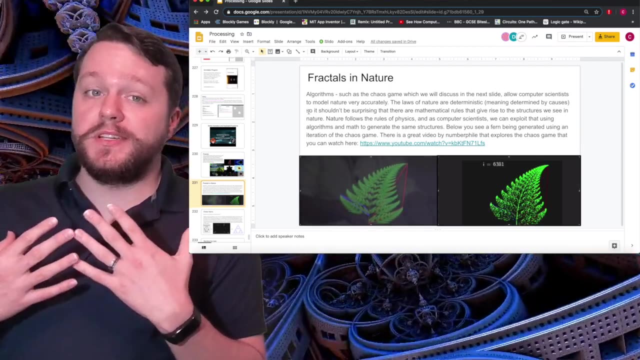 determined by causes. So it shouldn't be surprising to us that there are mathematical rules that give rise to the structures we see in nature. Nature follows the rules of physics and, as a computer scientist- not myself, I'm not a computer scientist, I'm a high school teacher- but computer scientists can exploit this using algorithms and 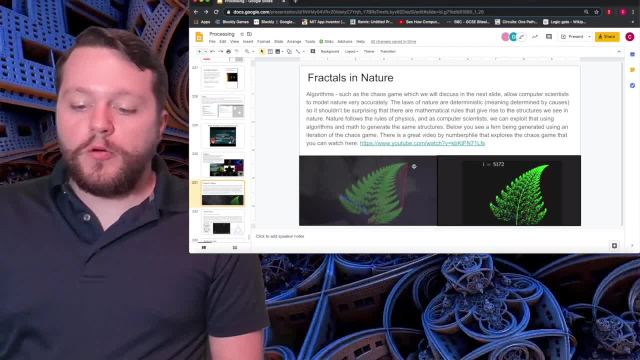 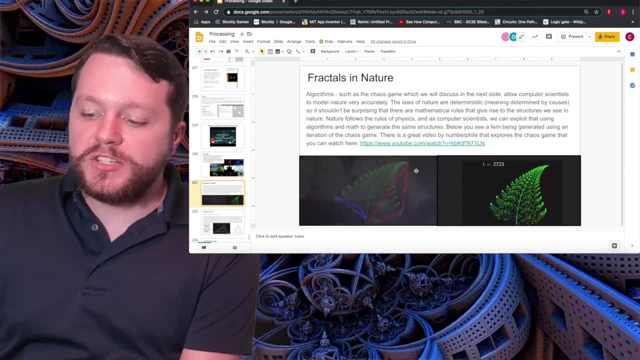 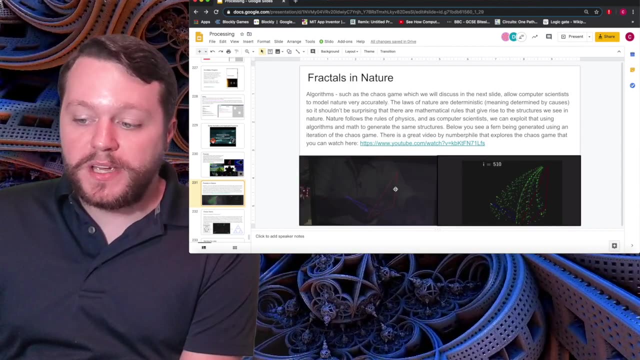 mathematics to generate the same structure. So a really interesting thing about the chaos game is that it has a huge element of randomness to it And yet the structures are kind of hidden inside of this randomness. So let's look at that in just a second. So this fern is being generated using a different way of doing the 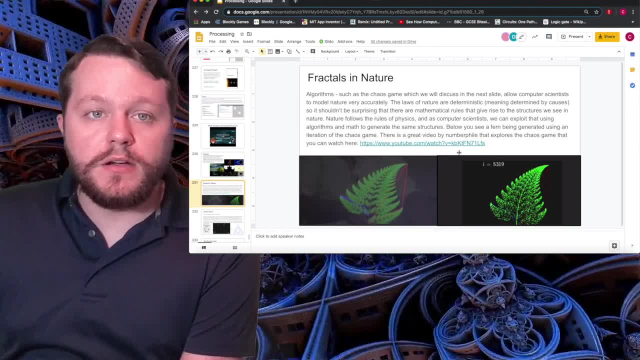 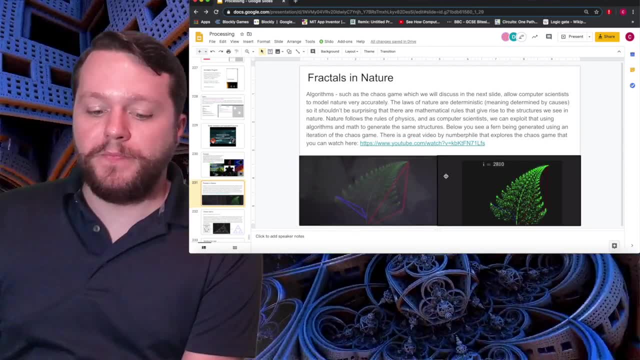 chaos game And, by the way, this comes from a really interesting video by Numberphile which you all should check out. So just in YouTube search Numberphile chaos game and it should come up. I highly recommend it. It's really cool. 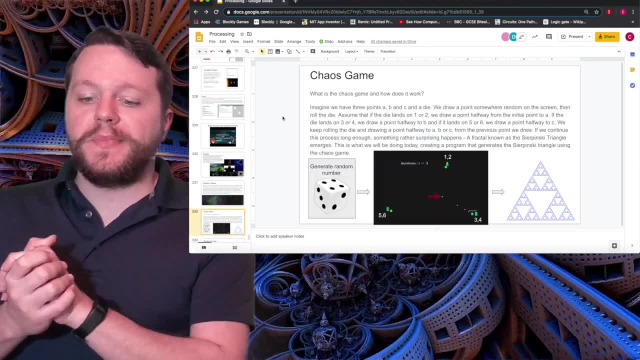 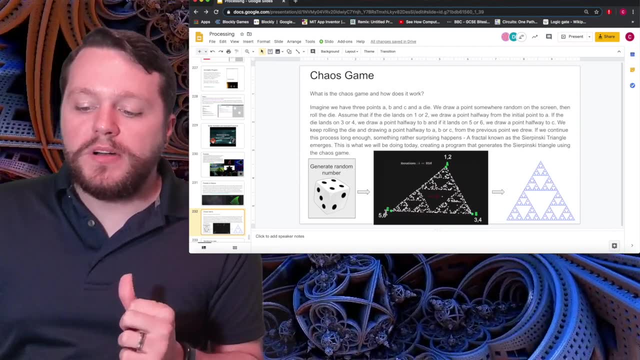 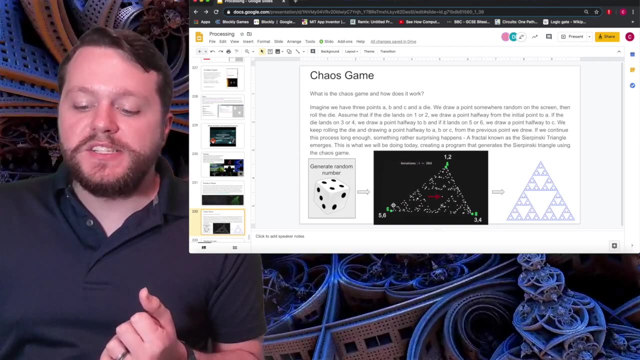 So what exactly is the chaos game And how does it work? So imagine that we have points A, B and C And we'll assign them some values. We'll say that A is the numbers one and two, B is three and four, C is five and six. 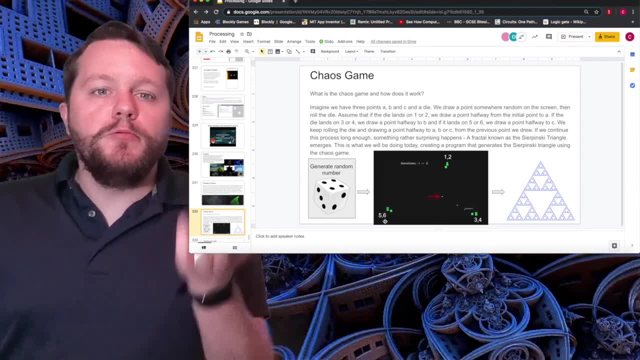 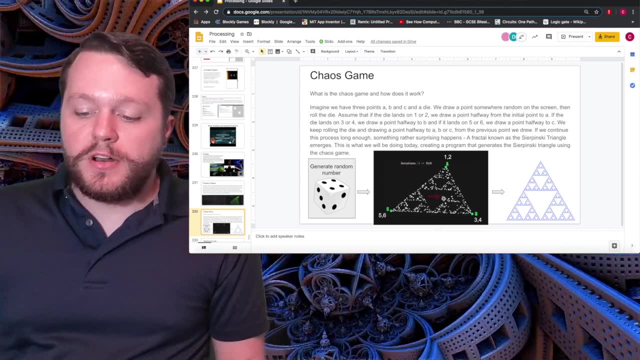 And then imagine we have some dice- just a single die, and we roll it. First off, what we're going to do is we'll start a point randomly anywhere near the triangle- This person started it right here in the center- And let's say: 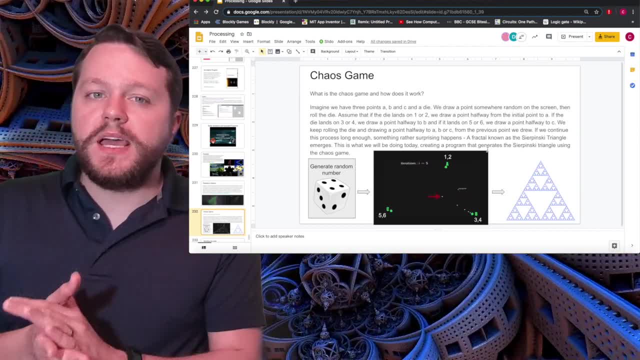 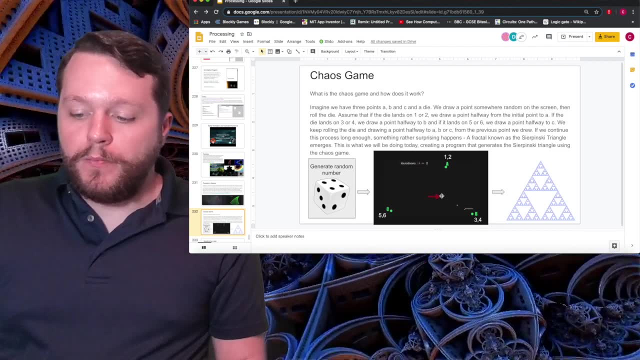 that the die lands on three. So the way that the chaos game works is that you then draw a point halfway from the point you were just at, one to the um, one of the vertexes, vertices. so b has three, four, and i said that the die landed on. 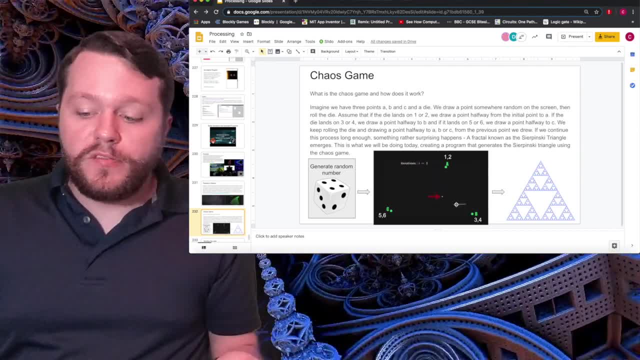 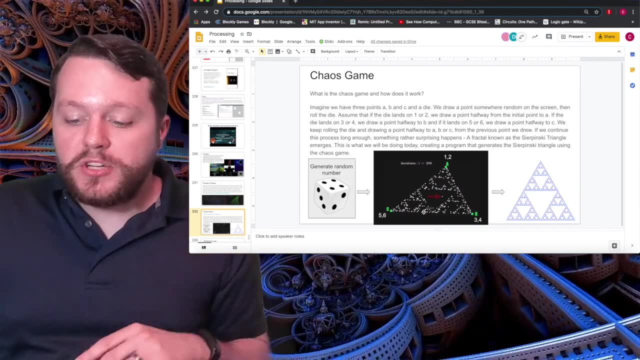 three. so we would draw a point halfway to three, roll it again. maybe it's four, move halfway to b, again, roll it again. maybe it's six. so we move halfway to c, and maybe it's a two the next time. so we go halfway to two, and so on, and as we iterate, this process for more and more and more. 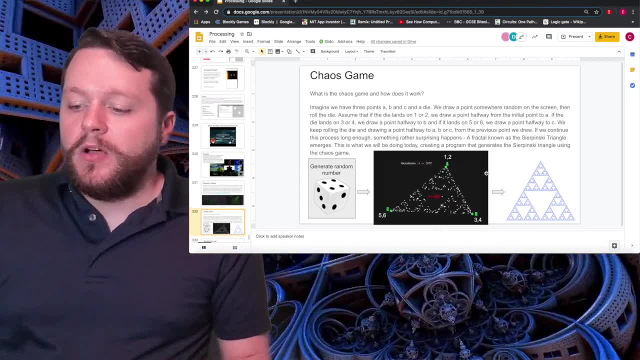 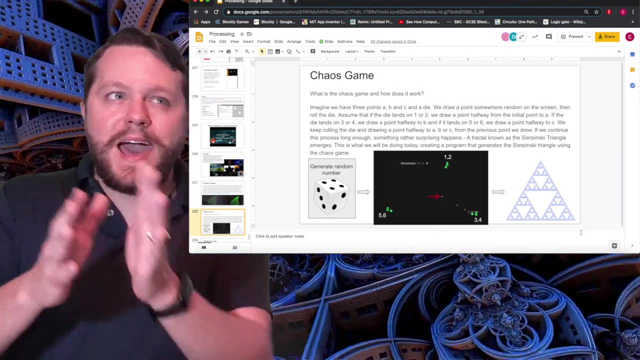 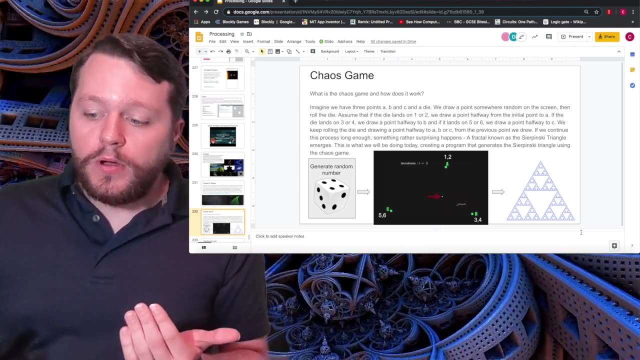 points, we get a really surprising result. this fractal called the serpinski triangle is generated by this half sort of random and half algorithmic process, so that's it's really surprising that this would even happen. what's really cool is that all of this is just nestled inside of randomness and 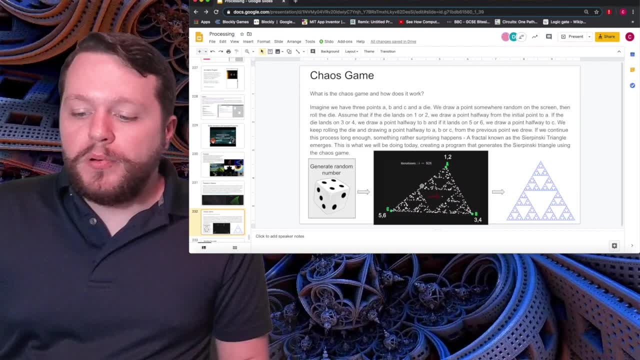 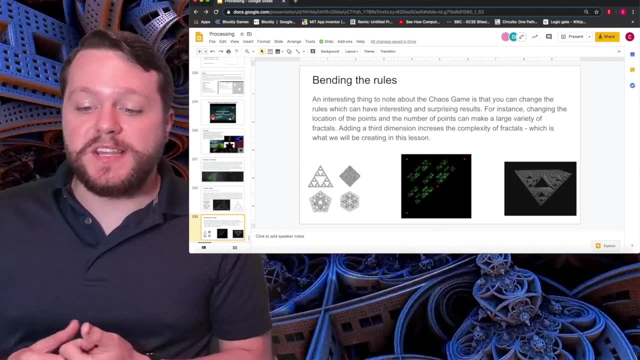 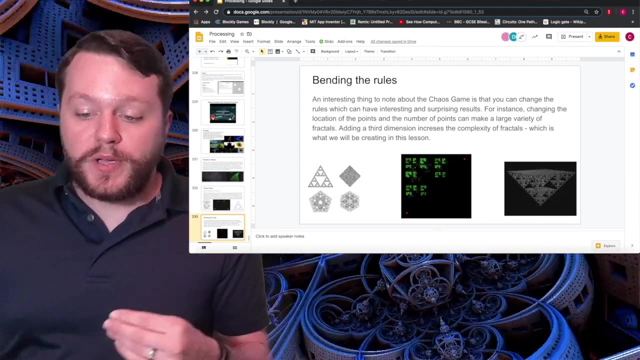 i think that's really awesome. by the way, we can play with the rules of the chaos game, so let's bend the rules a little bit. an interesting thing to note about this is that you can change the rules, and this has interesting and some surprising results, for instance, changing the location of the points, and you can see that. 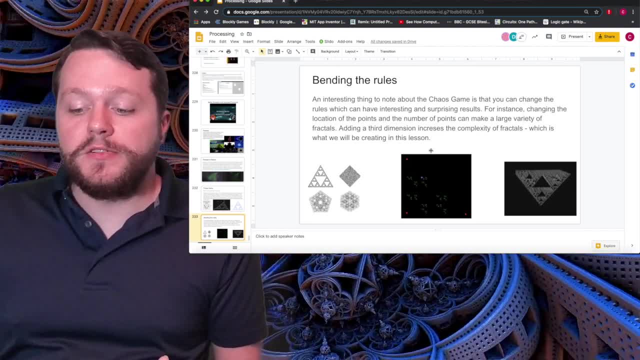 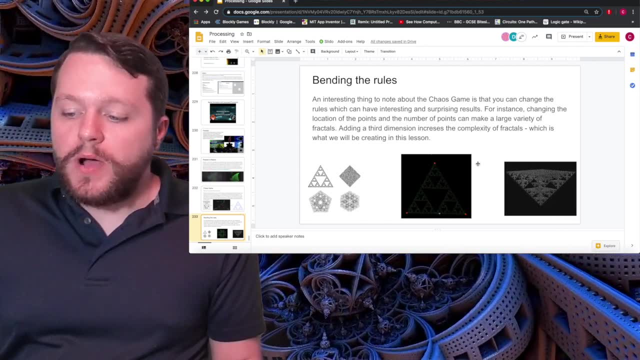 happening inside of here. as well as using a different number of points- see, they're using four generally- we only use three with the chaos game just to show that serpinski triangle and you can also add another dimension and, um, obviously, more vertices and have some more. 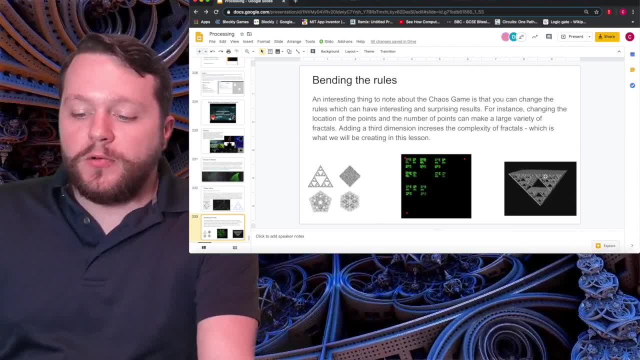 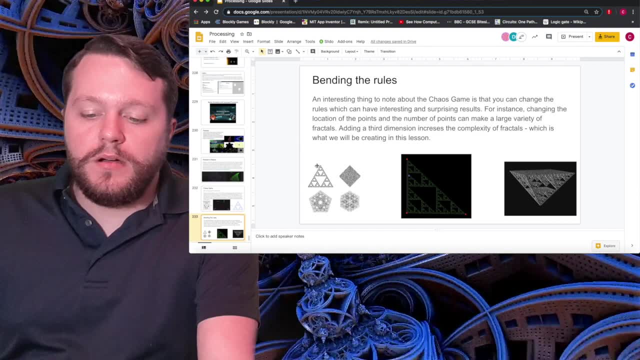 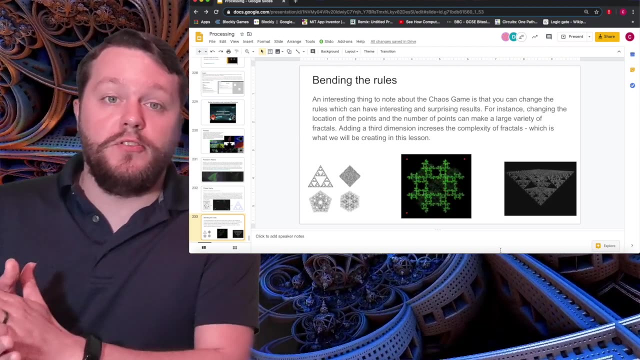 interesting results. so here's a 3d frame fractal. here we have points being moved um, different numbers of them, and then the way that you might draw or use the chaos game, with different amounts of points and specific positions, give us these interesting shapes. so, without further ado, let's make the chaos game. so i'm going to open a. 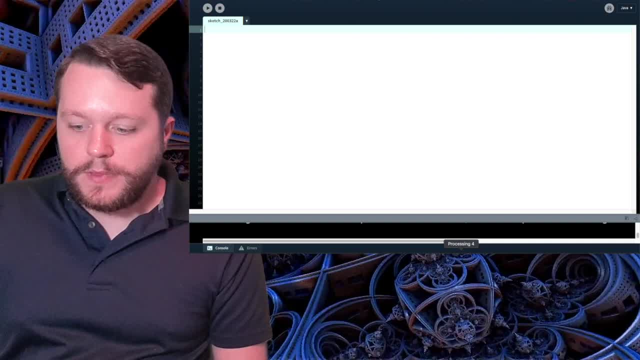 new project. oh, i hope i didn't leave the other one open, did i? if i did, i should pause that. okay, i didn't. i'm just going to close that. i don't need it anymore, so i'm going to open a new project. oh, i hope i didn't leave the other one open, did i if i did i? 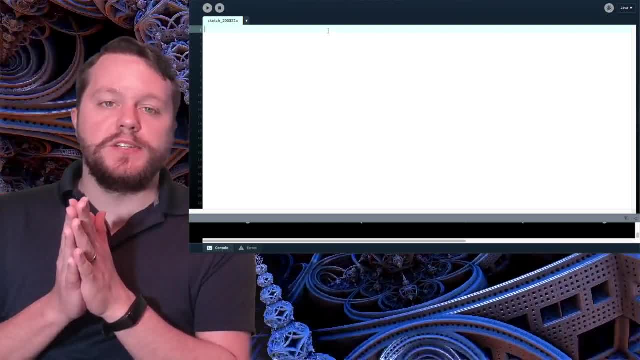 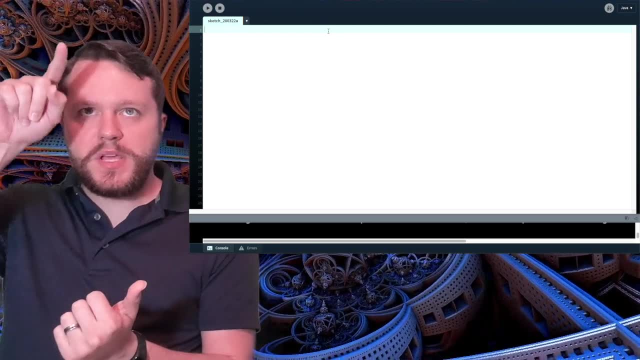 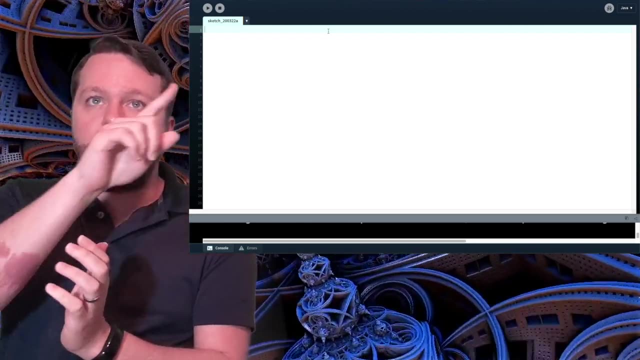 all right, so let's think about what the chaos game does. so, remember, we rolled a die to get a random number, okay, so we're going to need a random number generator. we have three points, um three vertices of our triangle, of just some shape, so we're going to need an x and a y value. 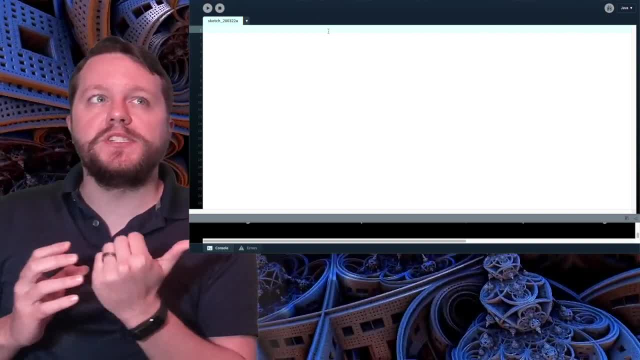 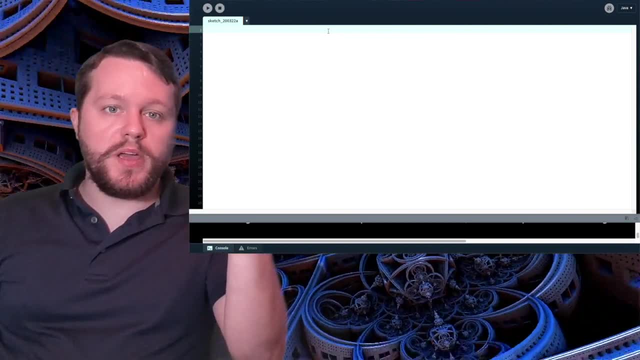 for each one, right? and then we need an algorithm such that, when that random number generator lands on zero, one, uh or two, the point moves half the time. so we're going to need a random number generator half way towards one of the vertices. so let's, let's make that happen. 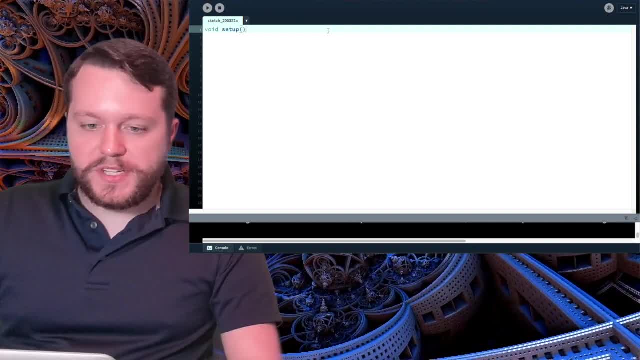 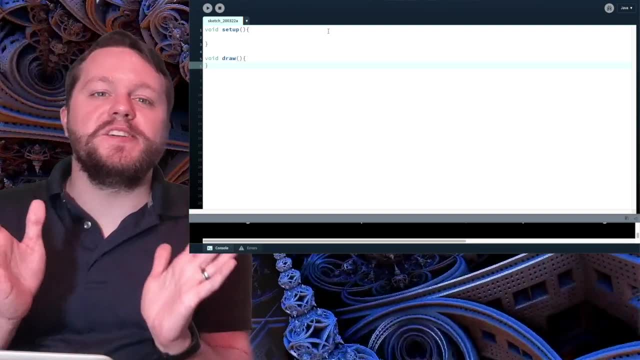 so i'll do void setup and void draw first, and, by the way, the first thing i'm going to make here is just a very simplified chaos game, and then we'll do a lot of the fancy stuff after that. but let's just see how the chaos game works. 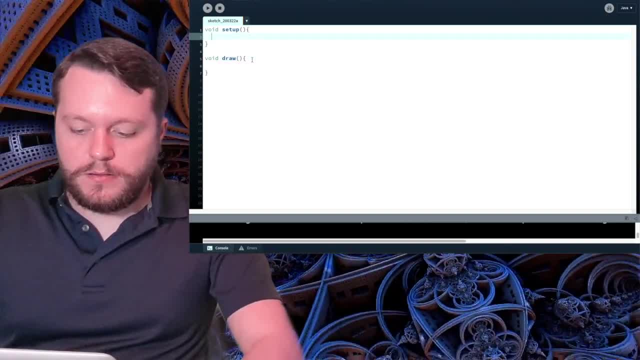 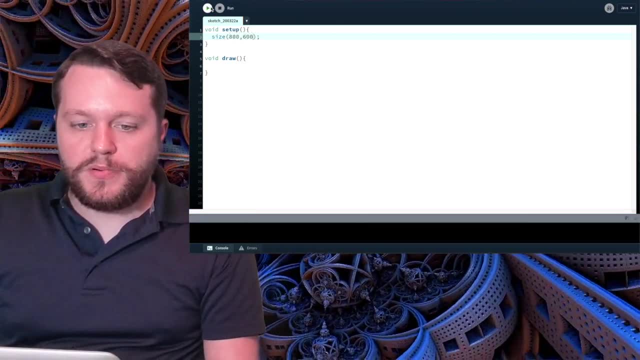 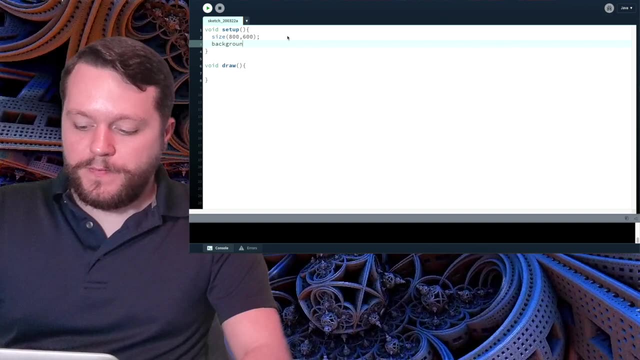 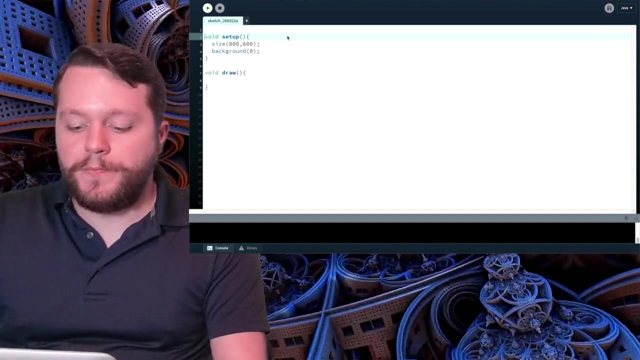 algorithmically. um, let's make it 800 by 600. that could probably be pretty good. nice, um, we'll give this some i. i like using black um for a background here now, so we need a random number, so i'll say float r, oops, and and this variable here. 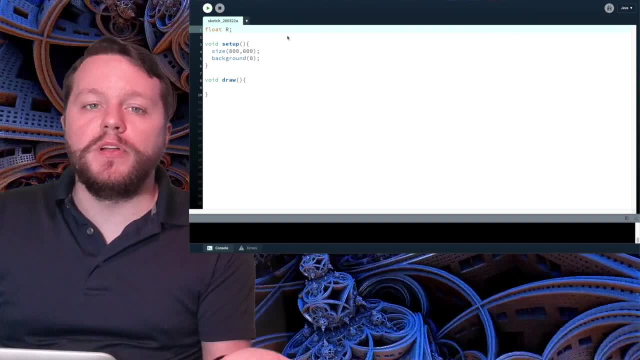 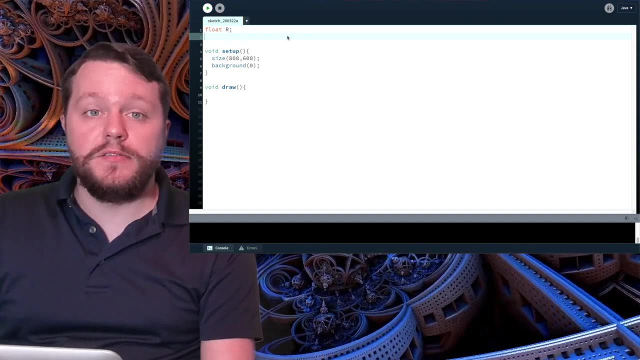 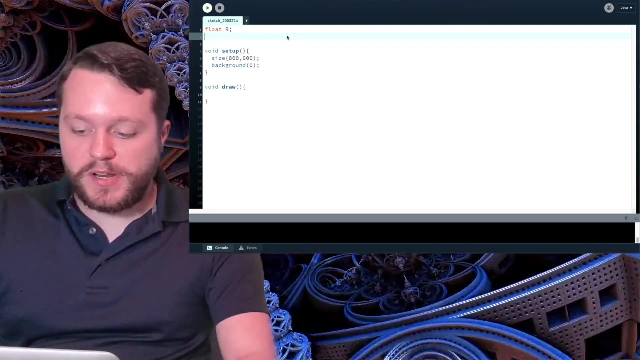 is going to store our random number, so this will act as our die rolling and giving us some random number to use. we also need the vertex of each or, excuse me, the horizontal and vertical position of each vertex. that will be our fractal, so i'm going to also make these random numbers float. um, we'll just say a comma b. 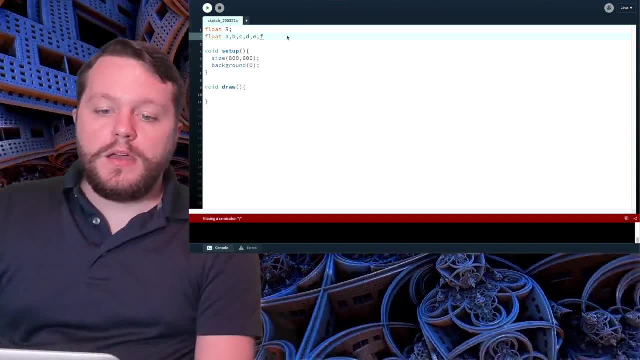 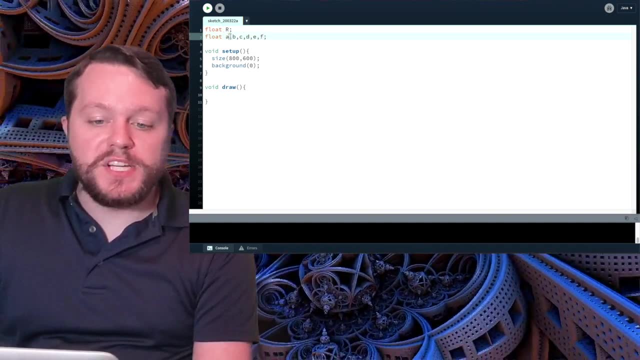 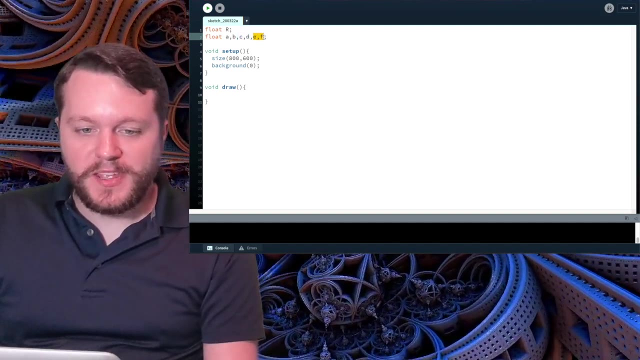 comma c, comma d, comma e, comma f. each set of numbers here will correspond to an x and a y position of each vertex of our triangle, our sierpinski triangle, um, and then we need a x and y position of the point that we're going to draw. 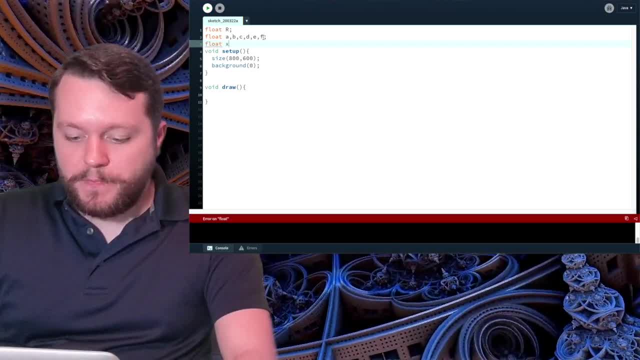 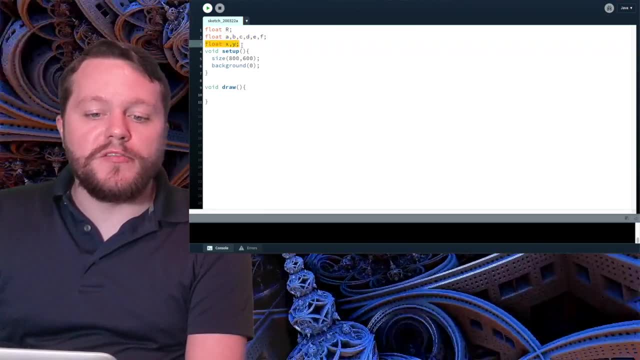 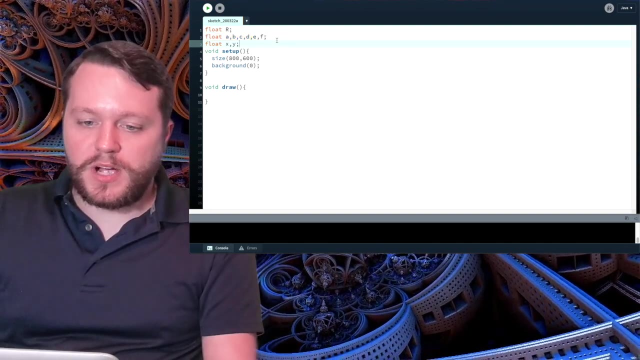 so i'll again say: float x, comma y, and the reason i separated these um in this way is i'm putting variables that are very related together, so that way it makes it easier for me to understand you know what variable is storing what. i guess i could also comment be like: uh, these are um vertex. 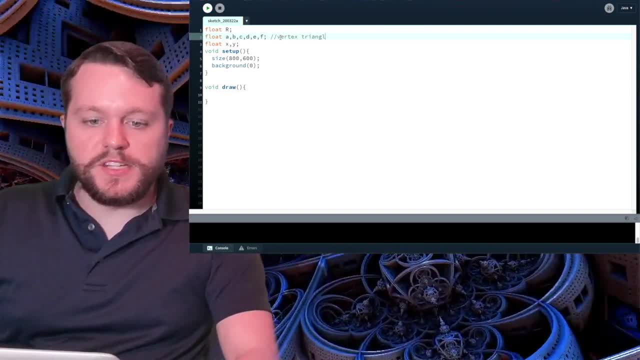 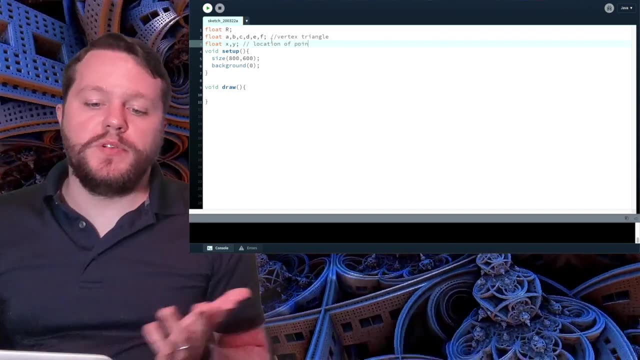 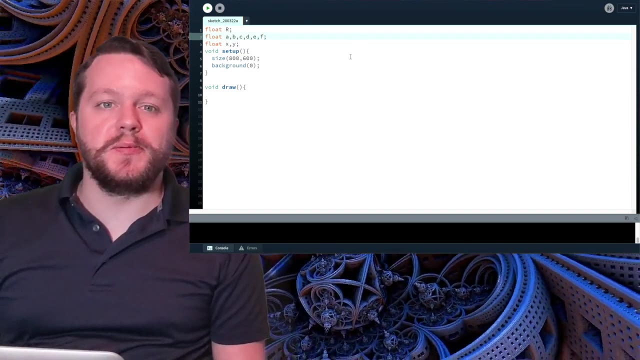 triangles, maybe this one, i'd say um location of point and so on. so it's really up to you how you want to do this. um, commenting is generally a good thing, but i'm i'm not going to do it, and that's okay if you don't either, but you should get in the practice of commenting, because it's really 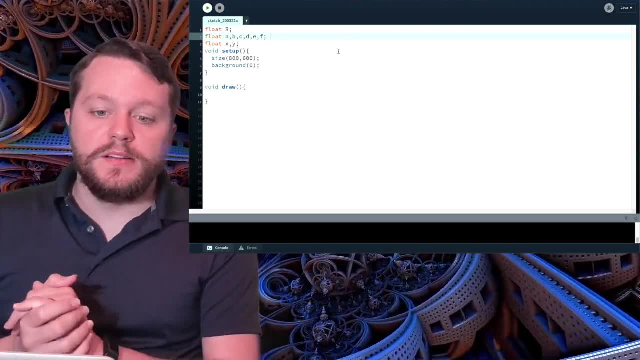 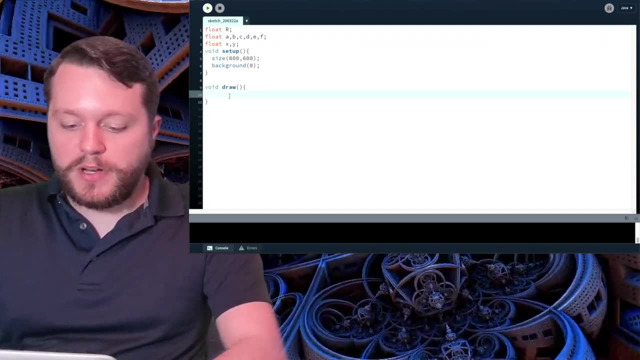 important as you develop your skills as a programmer. okay, so enough of me jabbering on about nothing. um, let's make the chaos game. so first, what we want to do is we want to do a lot of random numbers. so what we're going to do is we want to say r is equal to a random number. oh hold. 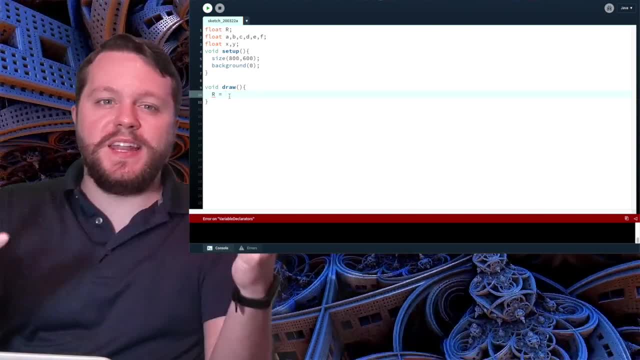 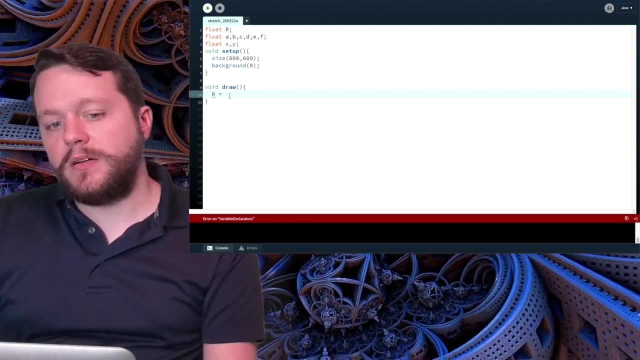 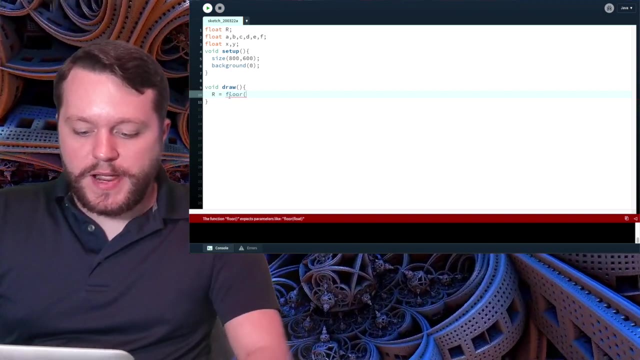 on, not just a random number, because the random function will just give us any float number. we want this to be converted to a number zero, one or two, um, so i guess actually i could have made that an int if i wanted. but it's fine, let's keep going. floor um of random of three, oops. 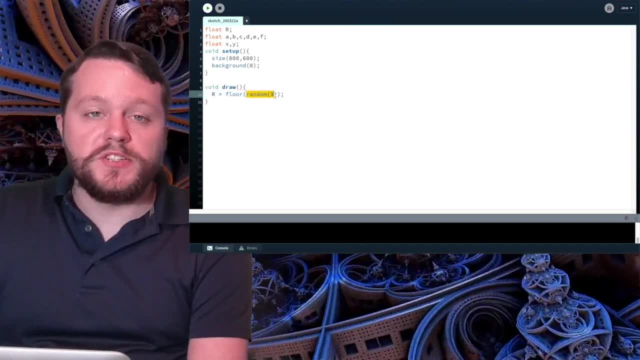 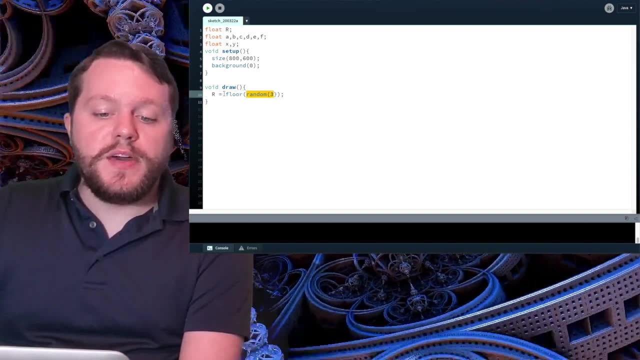 all right. so what this is doing is it's getting a random number between zero and in three and then, whatever that value is, it will almost certainly be a decimal number, a number with a decimal in it. Then we floor it to kind of lop off the extra bit, the decimals. 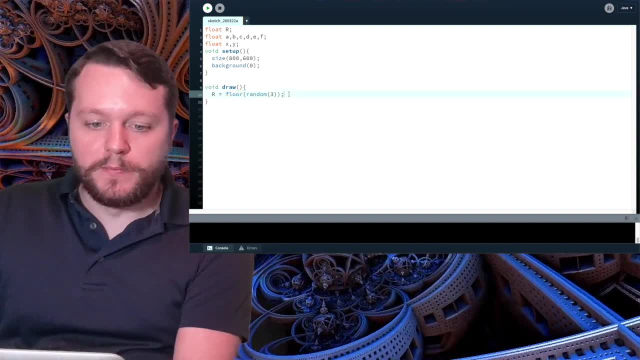 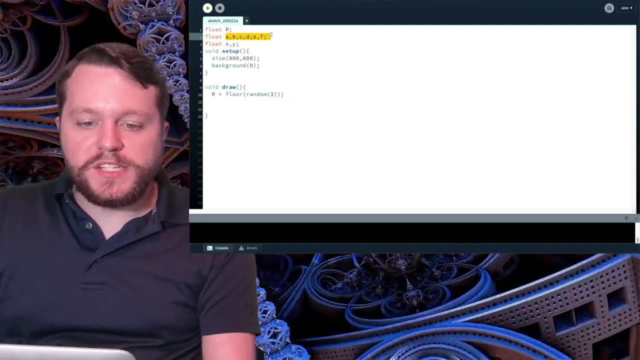 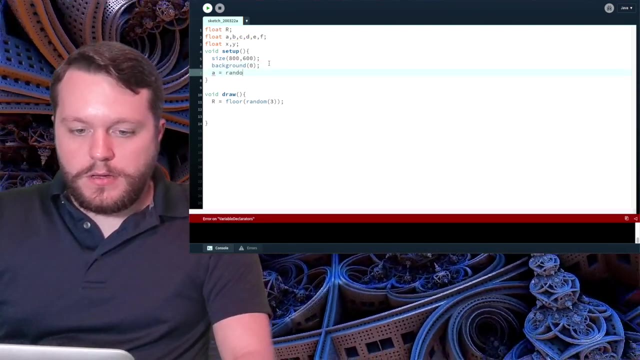 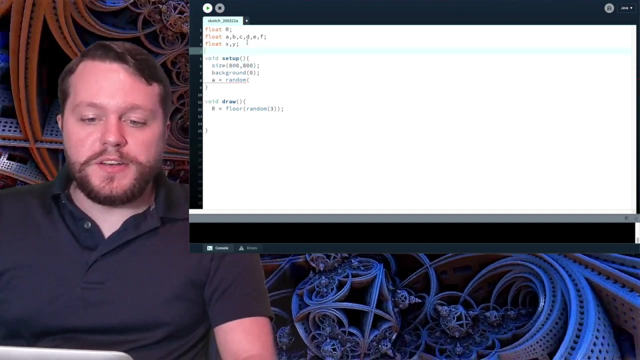 after it. All right, so that's going to give us our random number. Now we need an algorithm. Oh, you know what? Each of these need a position. So here I'm going to say a is equal to random, and let me change this from 800 and 600 to 800 and 800. And I'm going to make another variable. 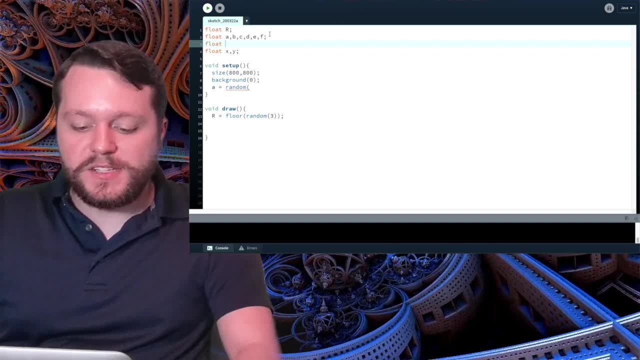 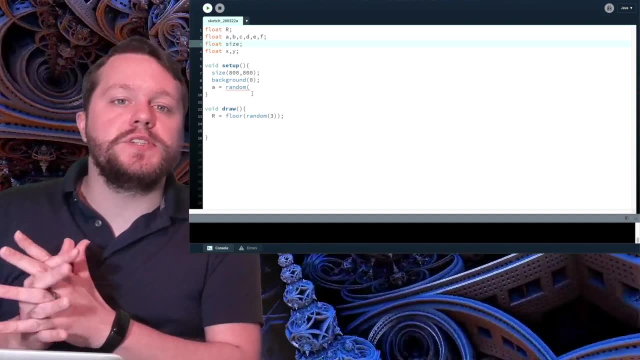 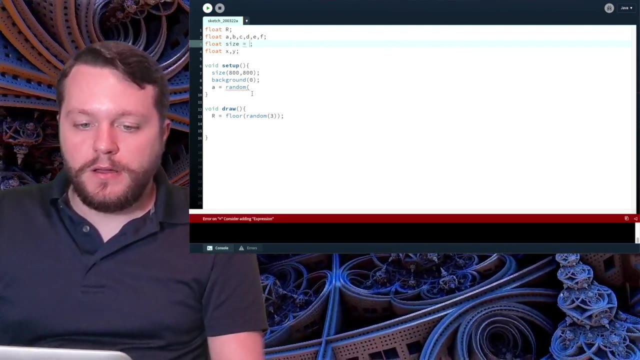 called size, And what this is going to store is the random. what value, between what values, a given vertex and x or y position of a vertex can be? So I'll set that equal to the width of the screen. Now, random in size. 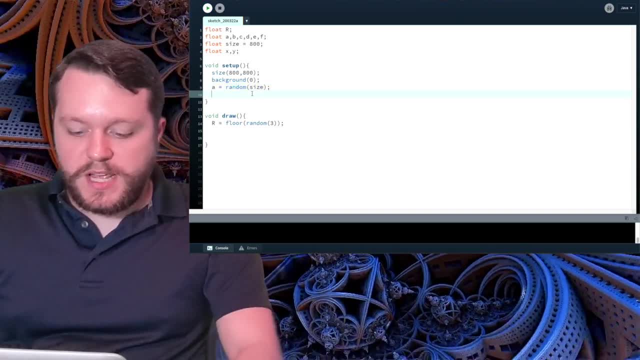 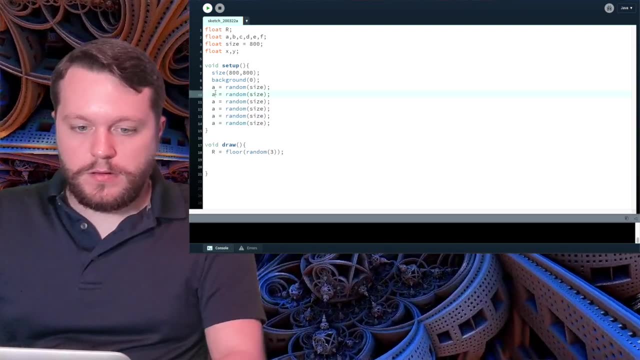 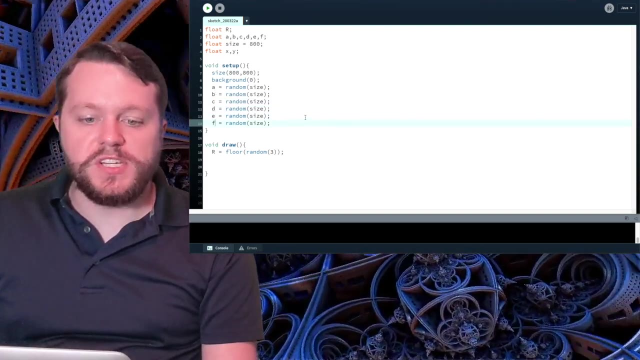 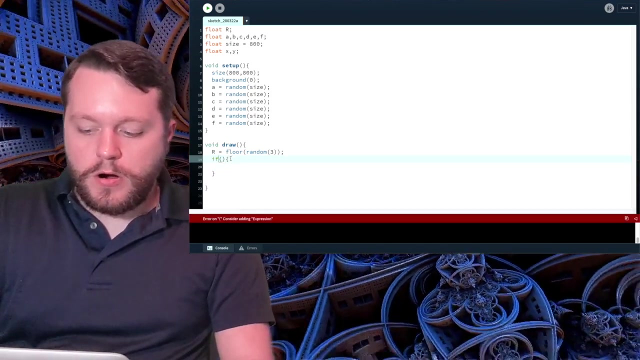 So this can only give us numbers between zero and 800. And so that's a, b, c, d, e and f. All right, so now we have vertices at random positions. Then we want to make our algorithm. So, if r is equal to zero, we want the position of the point, the horizontal position of the point. 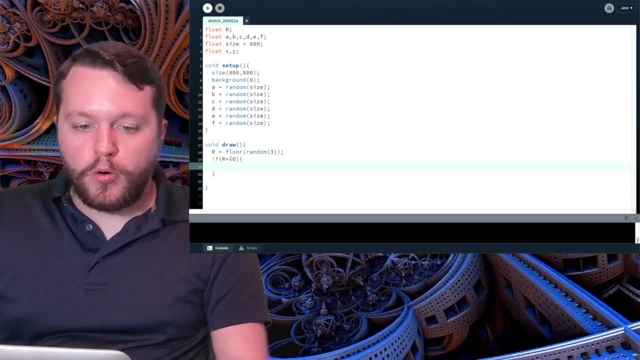 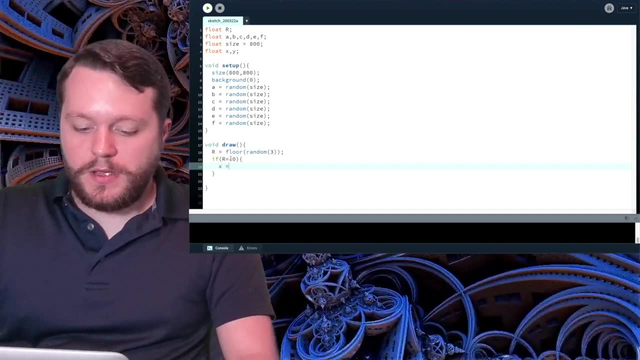 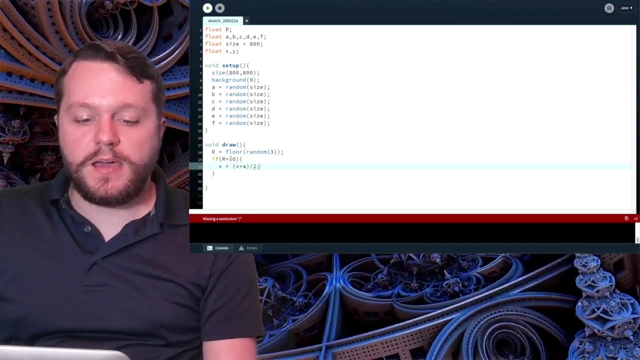 to be moved halfway towards the horizontal position of one of the vertices And we'll just use a. So we'll say x is equal to x plus a and then divide it by two. So we're halfway between x and a, And we'll do a similar thing for y, But instead of being halfway towards a. 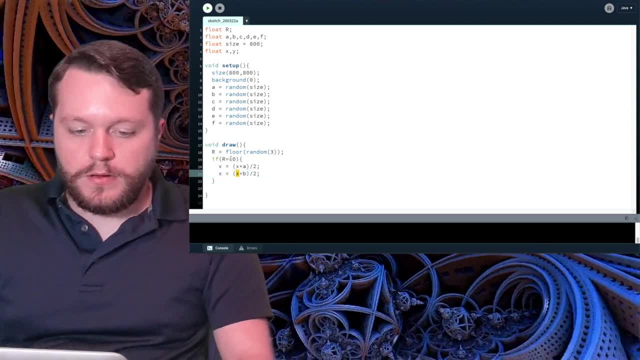 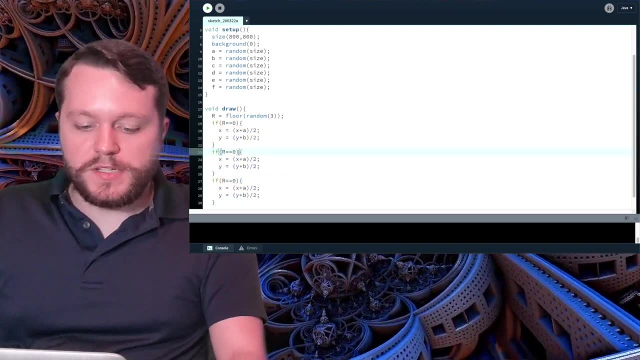 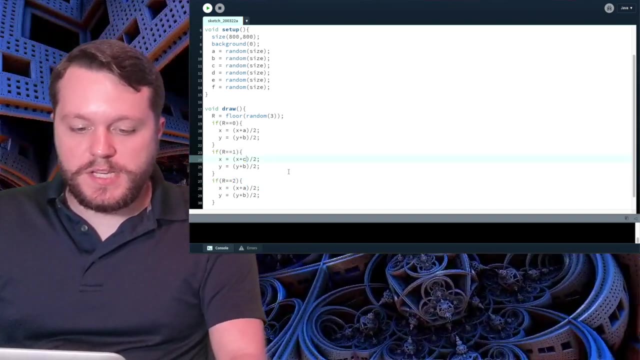 we're going to be halfway towards b, All right, And then we'll just do this two more times. So if r lands on one, we'll do stuff. If r lands on two, there's a, b. this will be c, d, e and f, And then we want to draw a point. 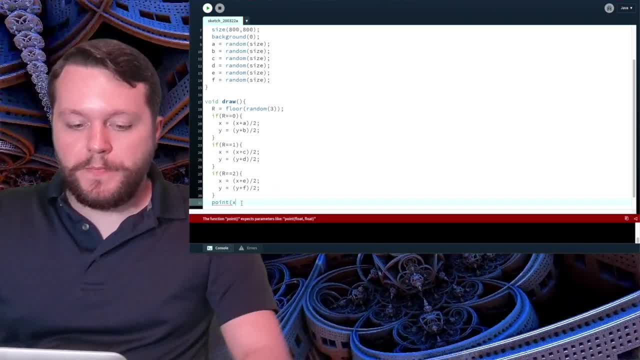 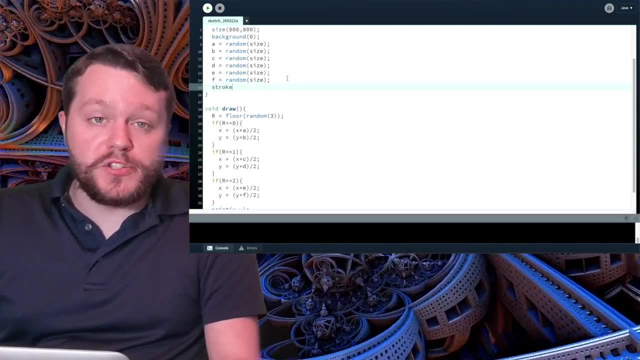 at x comma y, And we should definitely give the point a stroke value. If the background's black, the default value of stroke is black. So we want to make sure that we can see these points that we're drawing. So we're going to do this two more times And then we want to draw a point at x comma y. 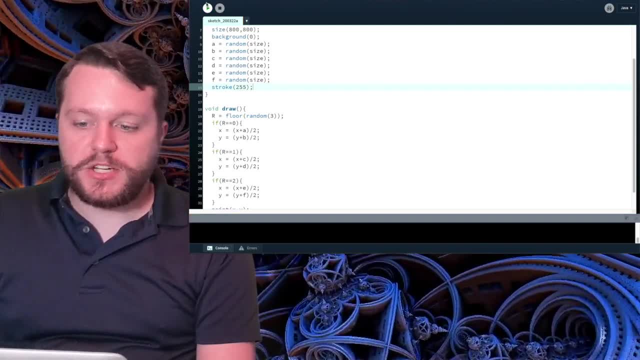 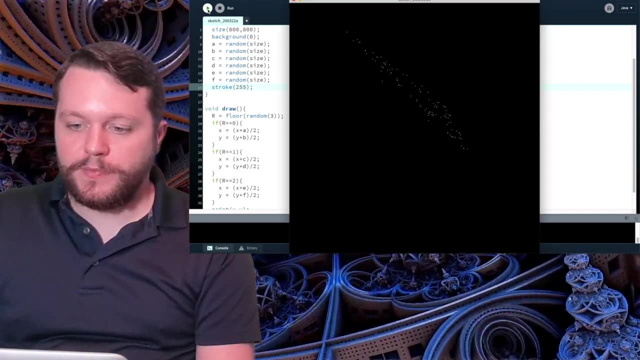 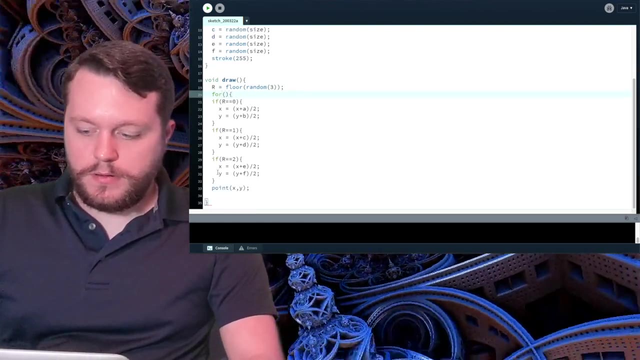 So I'm going to color them white with the stroke function, And that should be it. This is going extremely slow. Hmm, We can speed that up. Let's use a for loop. So for Oh, we need that to be in here too, because or else it's just going to. 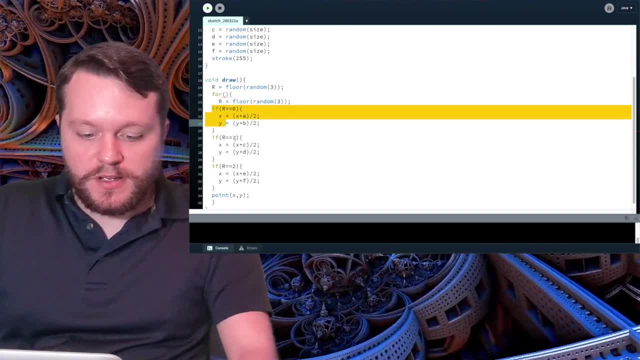 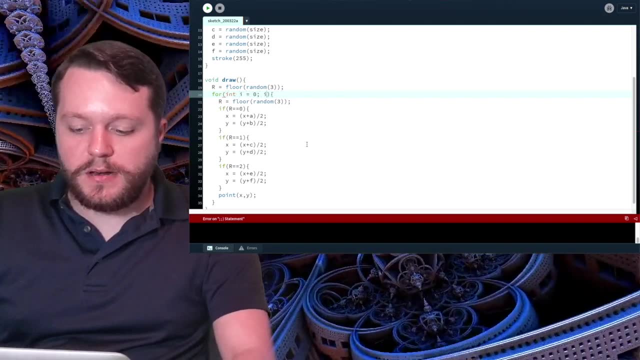 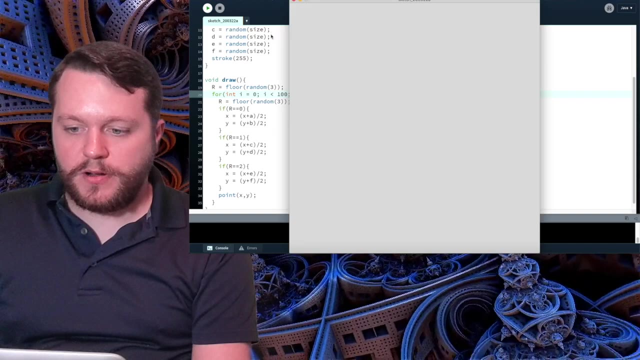 continuously draw points in places, the same places. All right, So for m int i equals zero. i is less than let's draw a hundred points per frame, i plus, plus, And that should happen very quick. That's cool, Awesome, And we can make it generate. 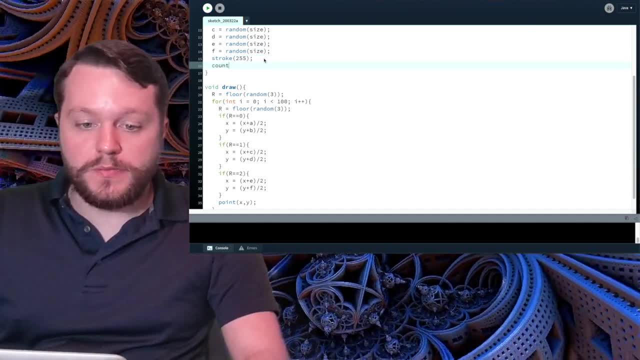 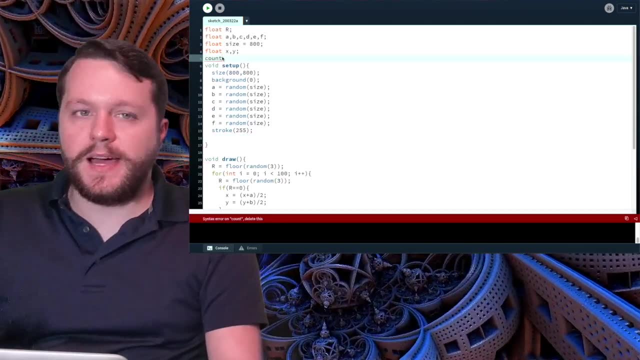 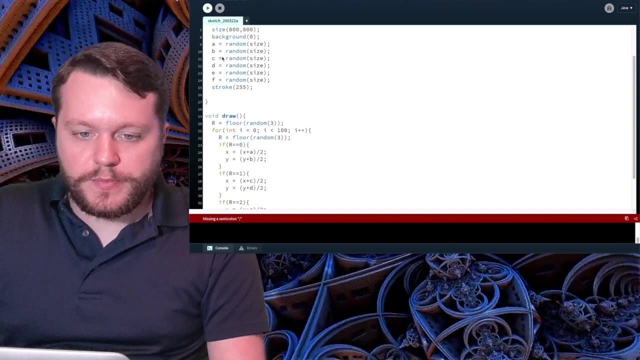 more and more random. Ooh, what am I doing? More and more random points or fractals. Well yeah, I guess you'd be generating random points too. So I'm going to make an integer called count, and it's going to be equal to zero, Yep, And we'll say count plus, plus if 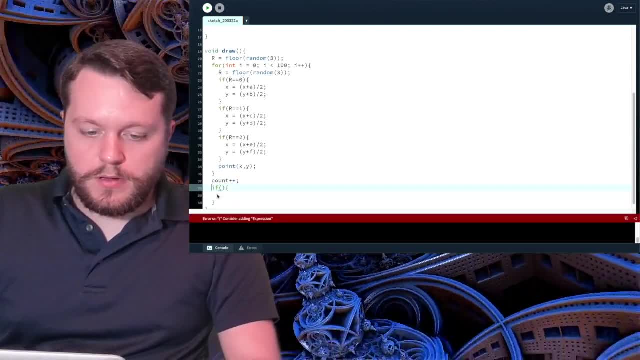 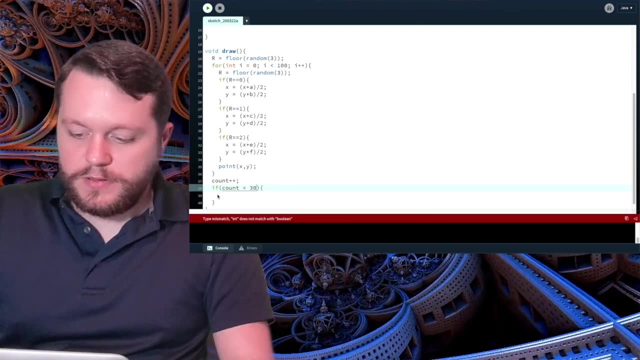 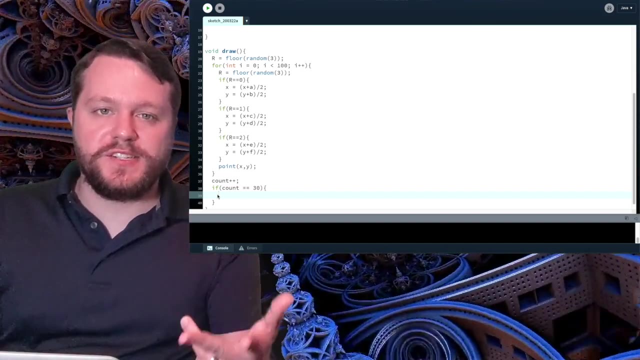 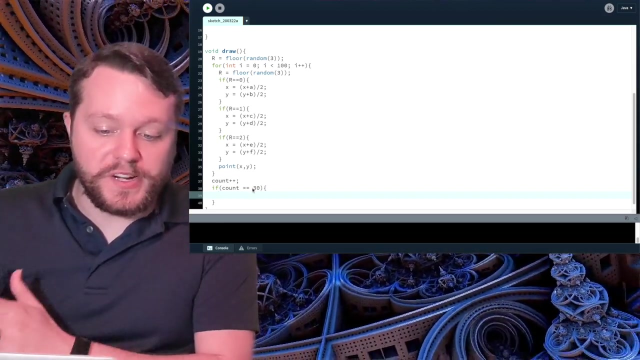 count is equal to 30.. Oops, two equal signs. One equal sign is an assignment operator. So we're setting something equal to something. Two equal signs asks. it's like asking a question: Is this equal to that? Um, all right, So if count reaches 30, we want to again randomize the positions of each point. 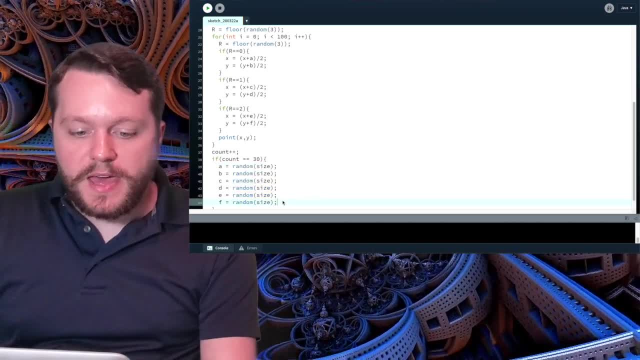 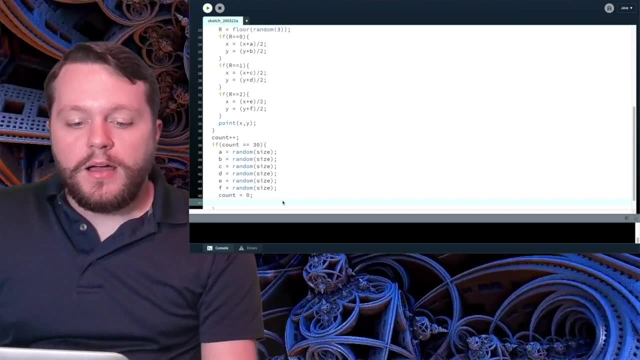 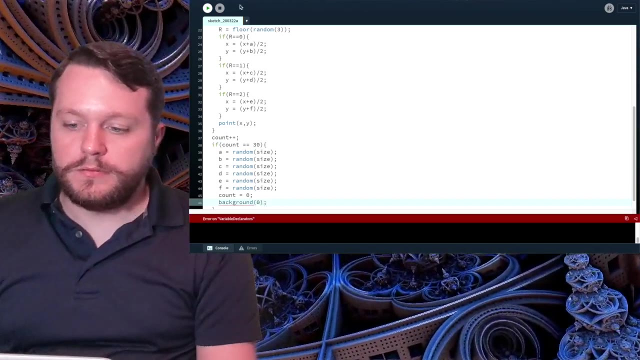 And move that over. And then we want count to go back to zero, So it just doesn't keep randomizing them forever. And then we want to cover up the fractal that we just drew using a background function. And there we go. So 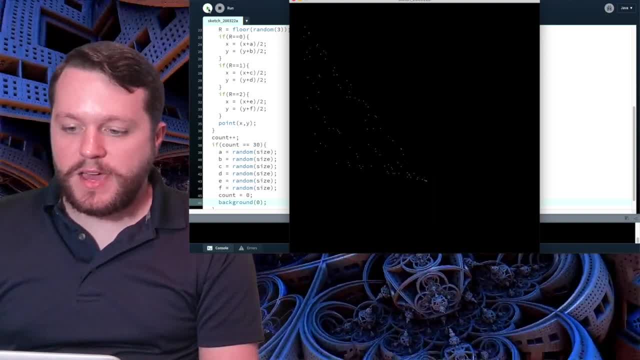 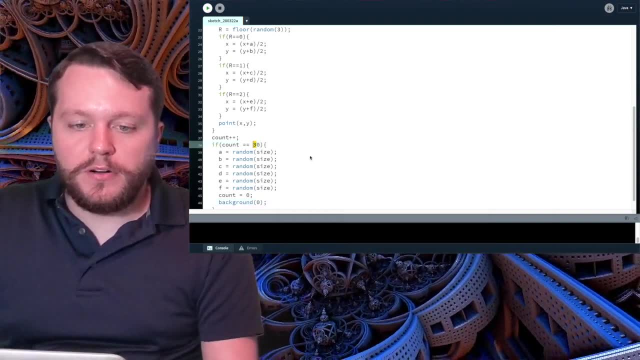 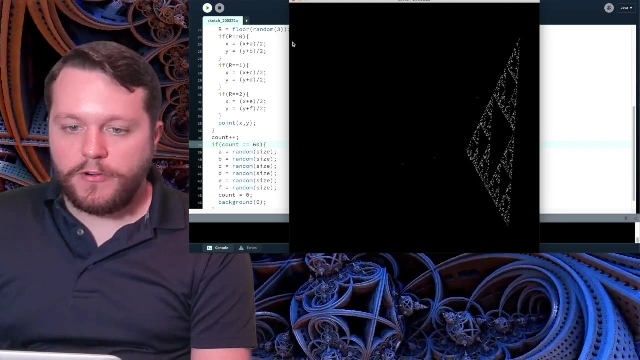 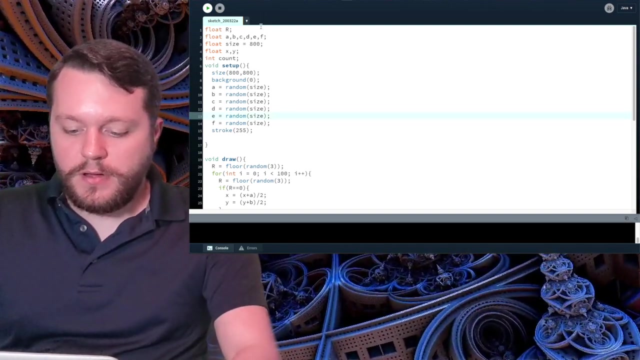 all right. Now we have a fractal generator using chaos game. That's pretty awesome And we can actually let it draw for a little while longer, maybe twice as long. For fun, let's add another point, So another vertex, to that shape. So E, F, maybe G and H. 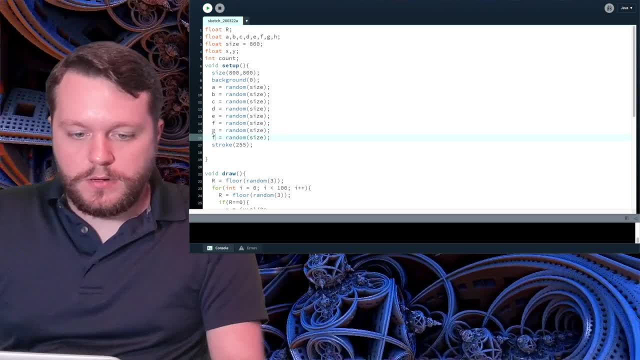 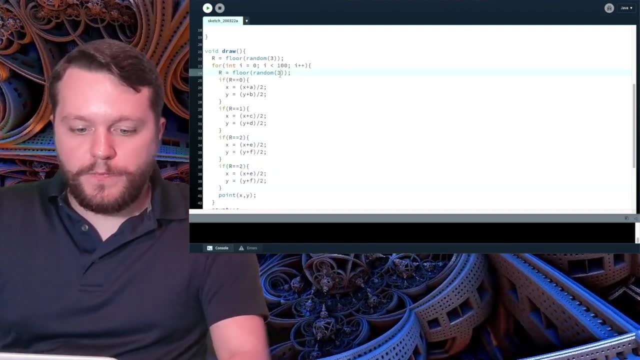 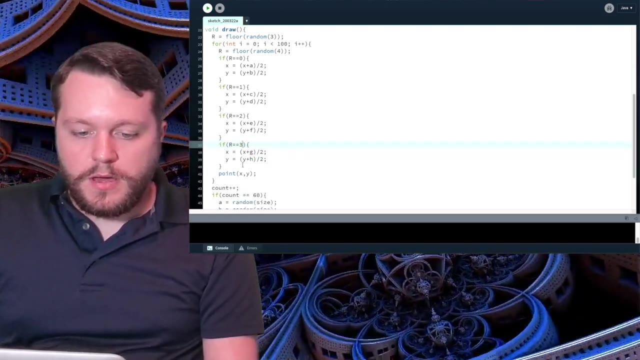 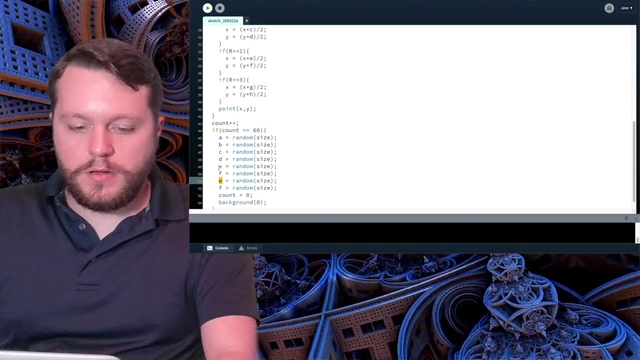 We need it to be able to the dice to land on G or H. Move that to four, G, H. If it lands on three, do stuff And Redraw its position. Cool, And now we have: Uh-oh, We're gotta go back to the last one. Let's make some changes, And I want to make sure I don't get lucky, But anyway, we're gonna go back, And then let's move it back to zero. We're gonna move it back to zero, So let's move it back to four. 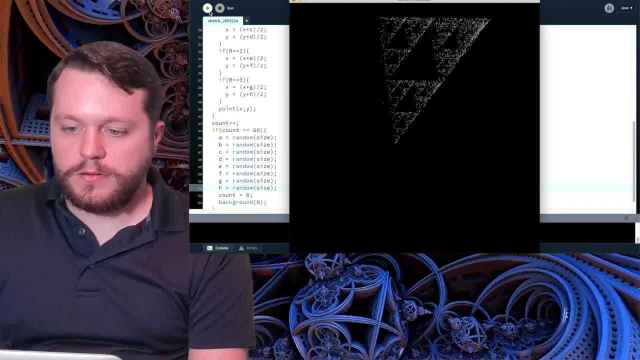 And then let's move it back to two, Because Andrea said they would finish this but we need to move it back to minus one, So we're gonna just move it back to three. Uh-oh Yeah, that's working Cool, And you can see that it's not quite the Sierpinski triangle. 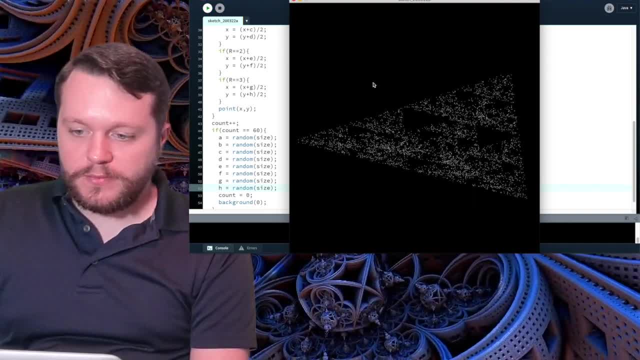 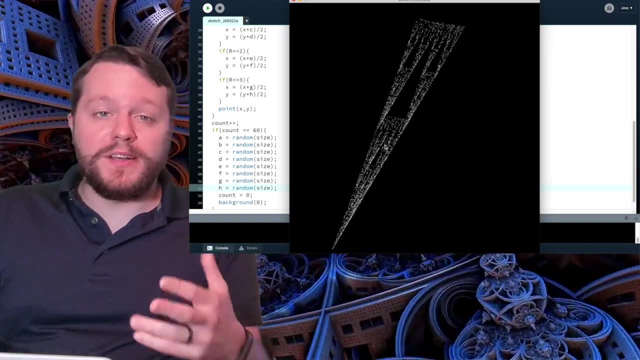 anymore. There's a little bit more going on. All right, so really we're done. So that's how we create the chaos game, using processing, What I'm going to do from now on. now, this wouldn't be for my students, this is just going to be for anybody who wants to learn how to make something a little. 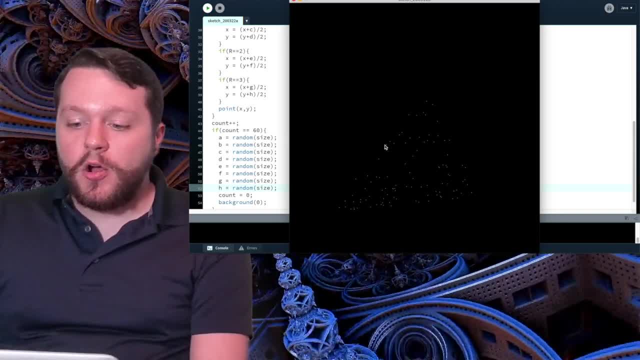 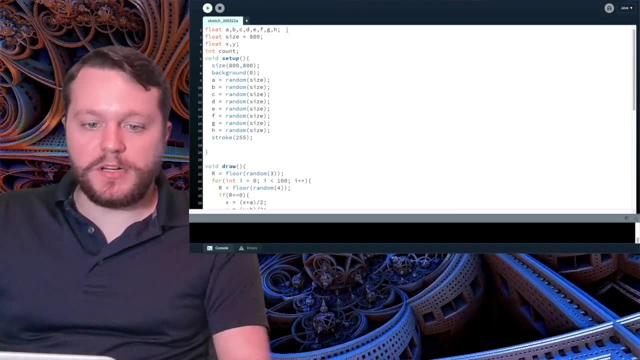 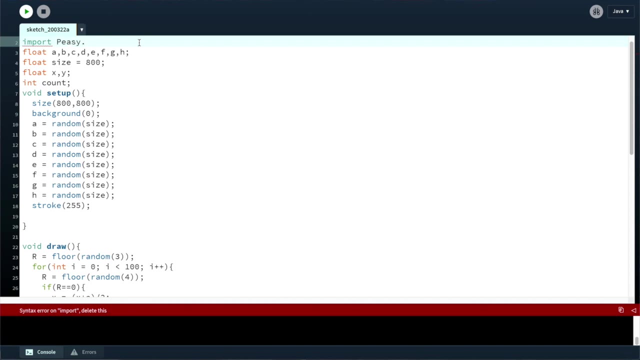 bit more complex and neat. We're going to make it so that we can move a 3D fractal around. So to make it 3D, first off, I'm going to need to import a library called pz Dot star, or does that need to be lowercase? No, that's good, All right. so importing a library. 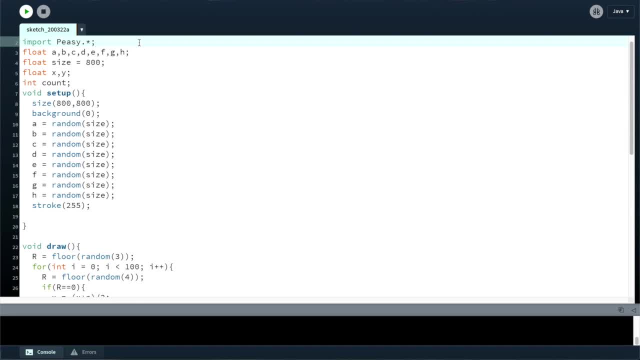 is something I haven't really talked about yet, but this allows us to gain access to more functions. that processing doesn't automatically start with PzCam. PZ is a library that allows us to do that, So we'll say PzCam and we'll make a very 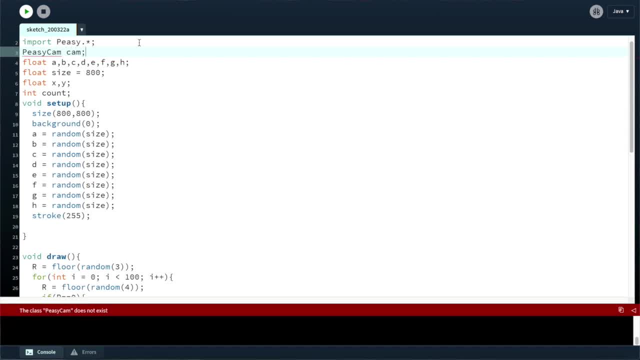 variable for the camera. Now, what do we want to do? Hmm, Oh Yeah, we need to make the screen have a third dimension, so we'll say P3D. Now, it's not going to look like anything is different here. Uh-oh, PZ does not exist. What are you saying? 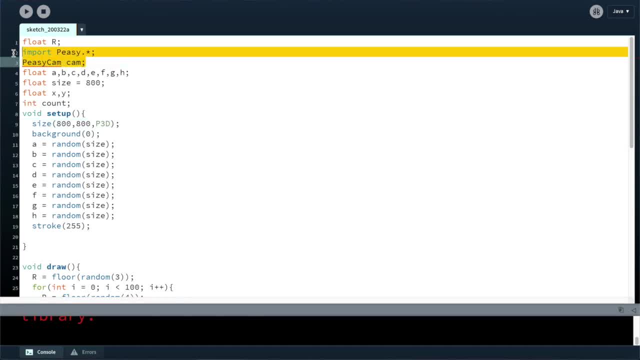 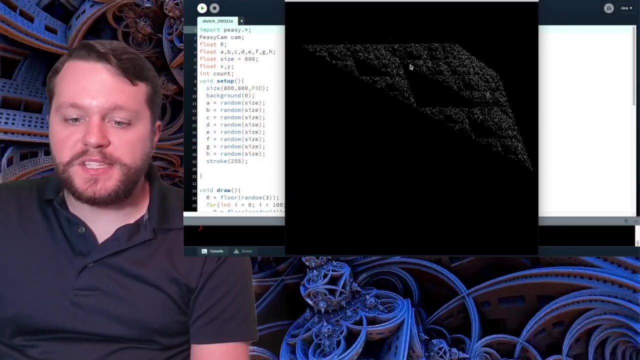 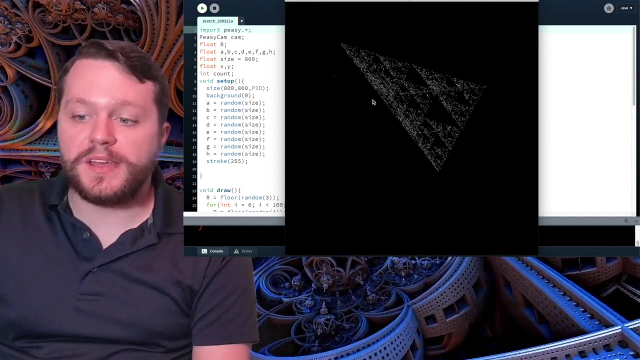 oh, it was supposed to be lowercase. okay, it wasn't giving me an error. that's weird. either way, we figured it out, so nothing is really different here. um, what we want to do is then use this variable to build a camera inside of this, so that way we can move stuff around. so to do that, i. 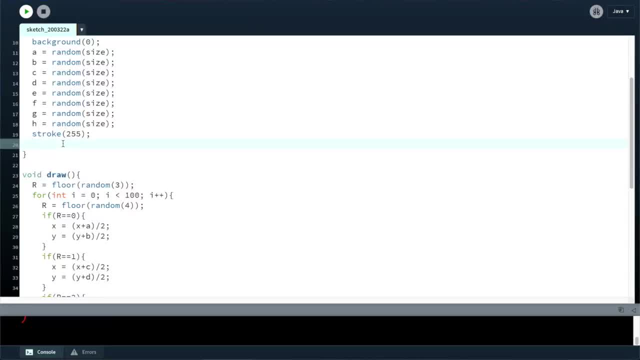 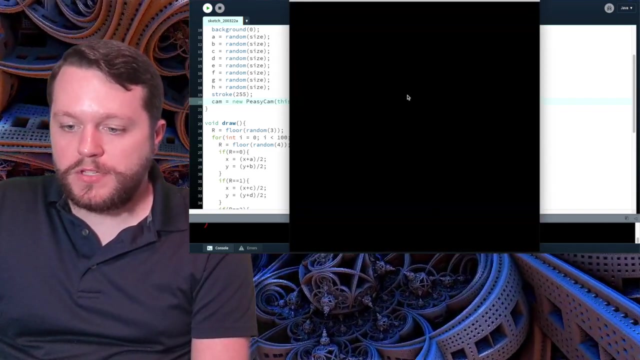 will go down here at the bottom of setup and say: uh cam equals new pz cam at uh, this comma 500, and now we should be able to move it around. so we just all that did was just invent a new camera. um, so one problem here is that because the background isn't getting deleted when i 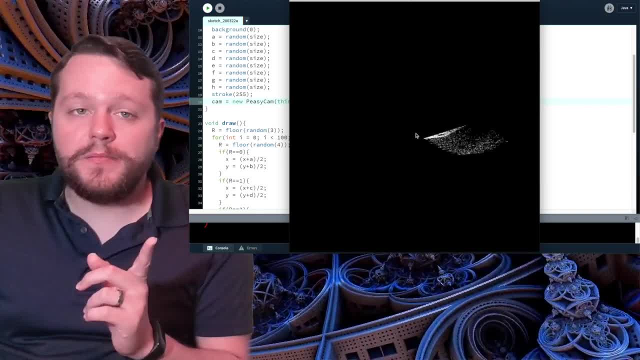 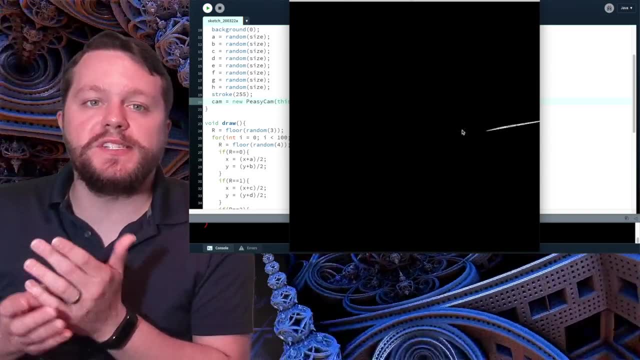 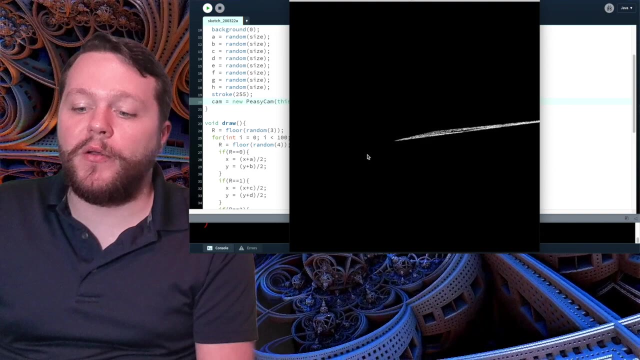 move this around, or, excuse me, i haven't made another background function and we can't really control all of these points, so what we need to do is we need to save those points into an array, um, so that way we can move the whole thing around and, uh, make the background. 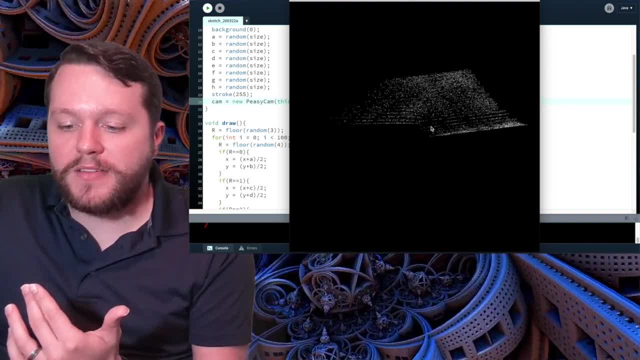 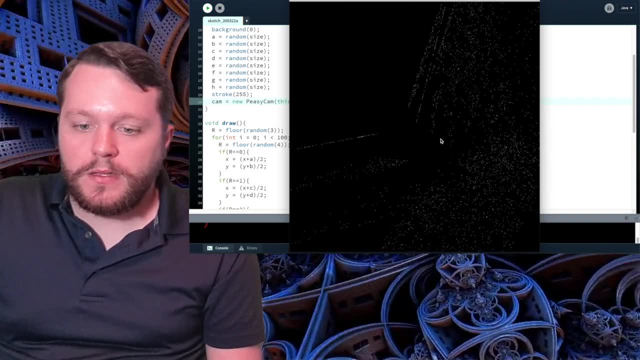 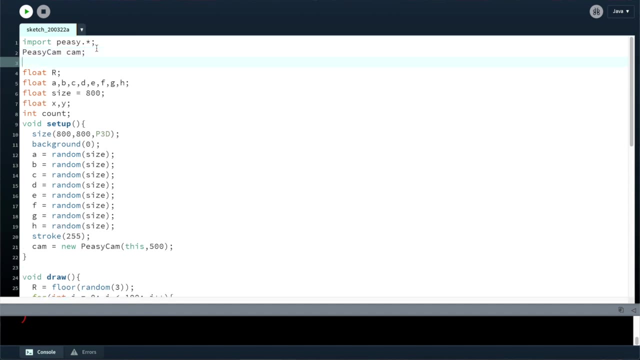 update, so it erases points and makes it look fluid and like what we want. this is definitely not what we want. it's kind of neat, but let's do something cooler, all right. so how do we do that? well, we need to make it array list um, say, array list um. 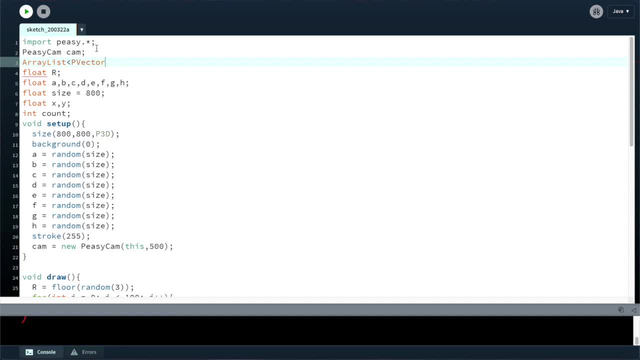 and a vector, by the way, is, uh, just kind of a direction in, and for us it's going to be in three dimensions. so because, if we think about this for a second, the, the fractal that we're going to be creating, each point of the fractal, 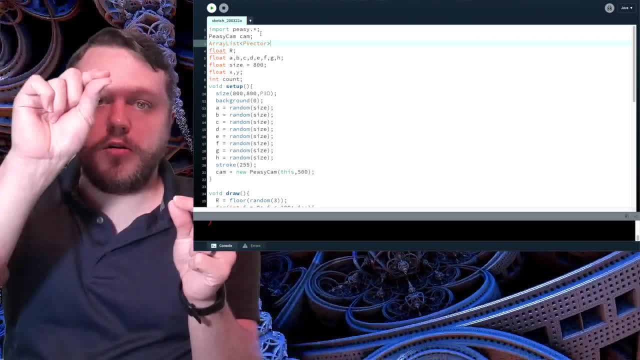 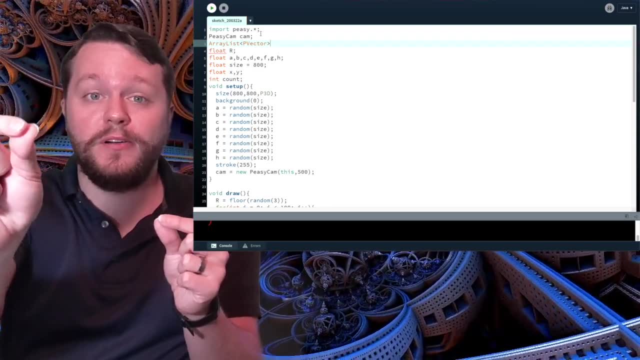 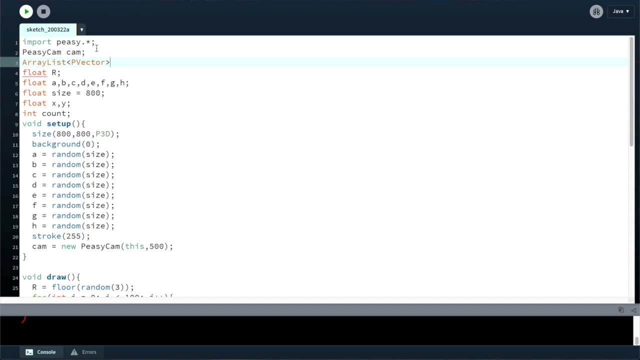 each vertex is in three dimensions, So we have to declare how far over, how far down and how far into the z direction we want this point to go, okay, So we're going to need to store all of those inside of an array list. So that's what I'm doing right here: New array list, and 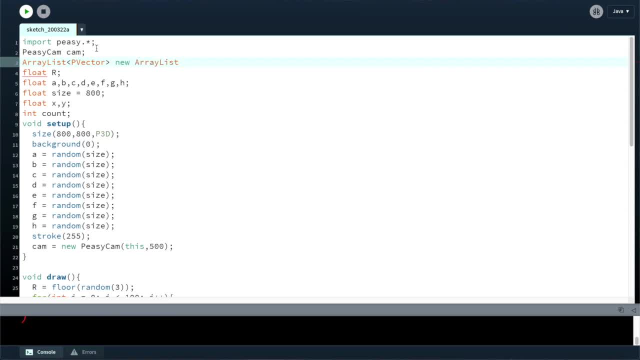 and that should do it All right. so there's our array. Oh, why do you hate me? What's wrong? Oh, it's got to equal that. Okay, we got it. Awesome. Now we need to store well. 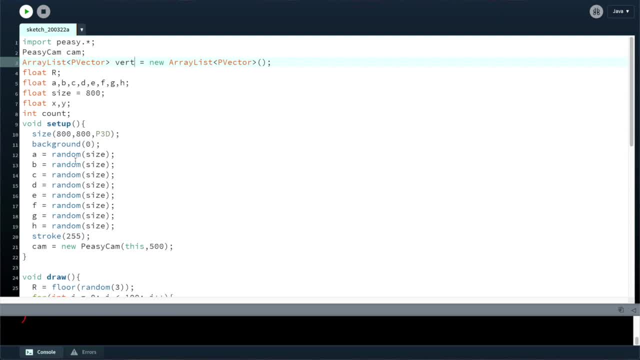 since each vertex of this shape is now going to need three variables to describe its position, we need to make some changes here, So this will be the first vertex, the second vertex and the third vertex h. I'm not going to use i and j. 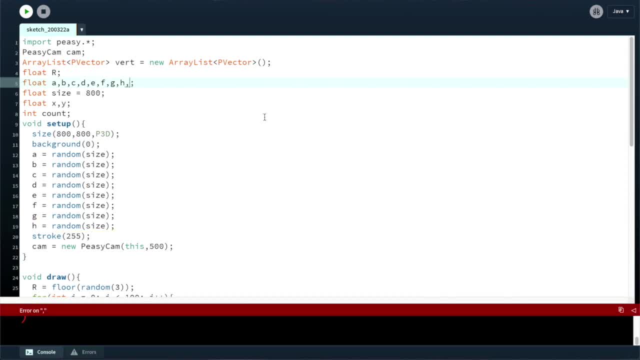 because I usually save those for for loops. So instead we'll say k? l is that enough? There's a point, there's a point, there's a point, okay m? n. So I want to do something more than. 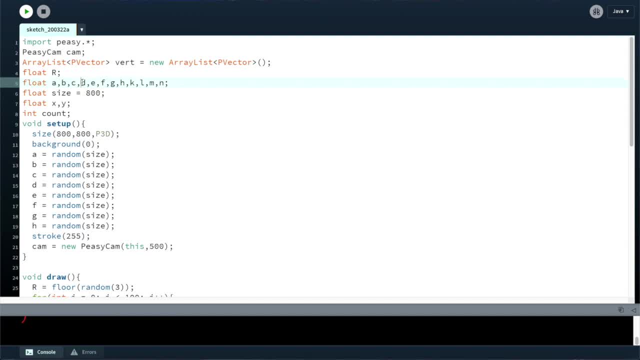 just have a fractal with three vertices. I think it's neater if it's got more. we can do some more exploration. So right now we have four points and we may add a fifth. So that's one, two, three. 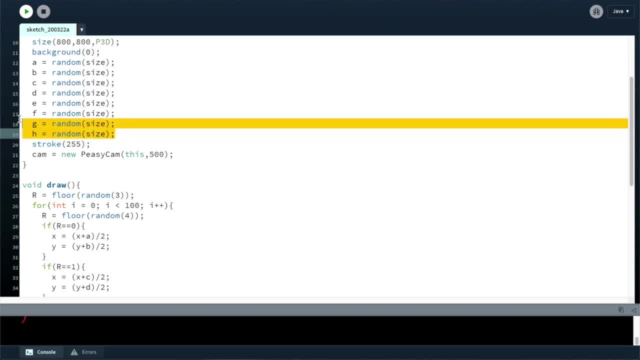 and four, We'll need to draw random positions. Okay, l, m, oh, I need one more n, is that right? Yeah, Okay, what is next? What do we want to do now? So we made it 3D. 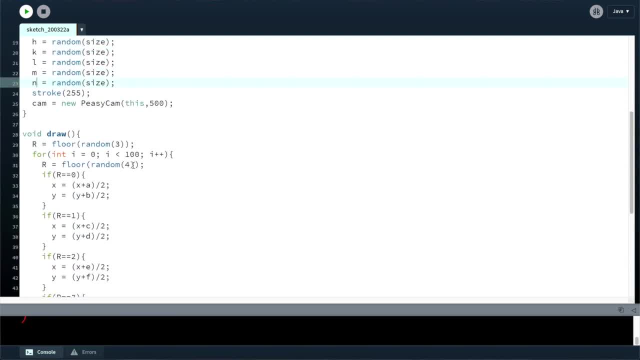 We made our ArrayList to store those points. So I'm going to do that. why did I leave that there? I'm going to do that here. So I'm going to say it's going to be a for loop And we'll call it v for vertex Invert, and then we want to draw the point vx comma, vy comma. 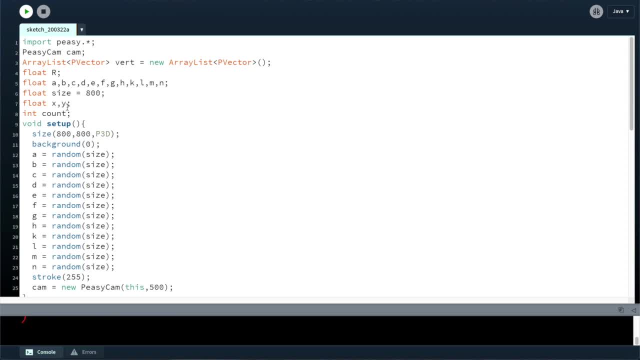 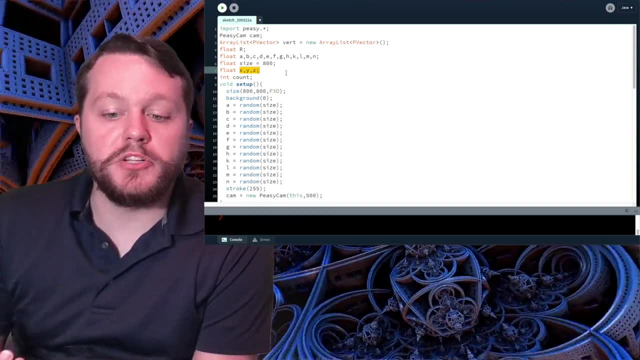 dot z. There we go. And I did make that z value right, I did not. So there we go, And this will be the location of each point that we've drawn this x, y and z position. So one thing that I. 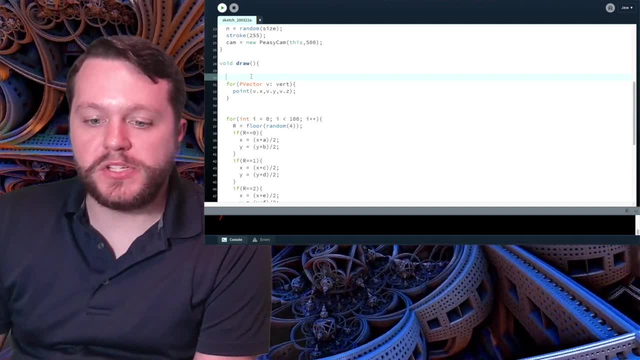 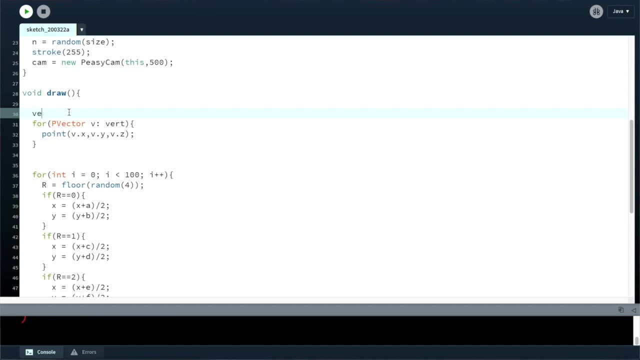 forgot to do above. this is we need to be able to add these points to that vector, but also draw them. So what I need to say is: vertadd, and within these we will say new pVector at x, y, z. 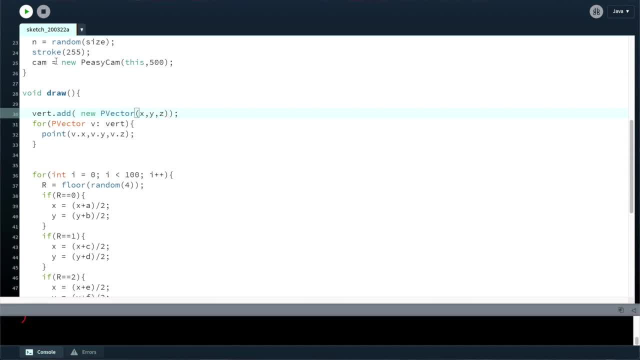 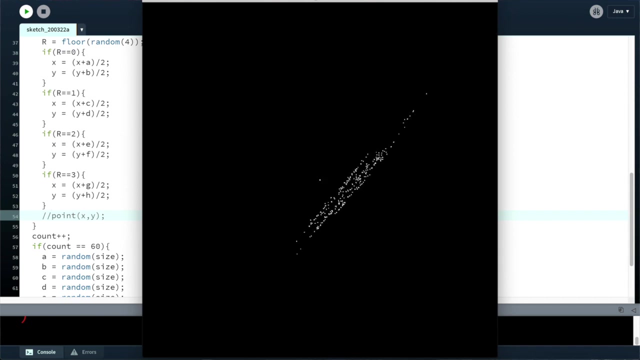 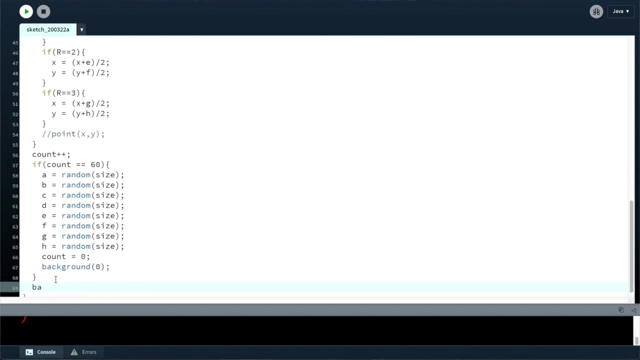 All this is supposed to go inside of some parentheses. There we go, Cool. Then we want to store them and draw them in a point. Well, it's still not. Oh, we didn't update the background, So I can just do that down here. 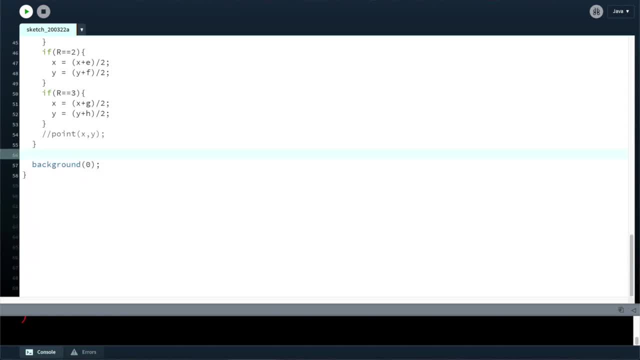 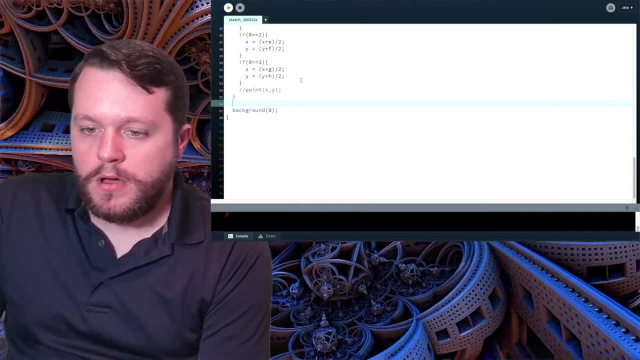 I'm going to get rid of this if statement because I don't really want it for what we're doing. So let's see: Did that work? Did we do it? Uh-oh, Oh, you know what I put background down at the bottom, So everything that we just drew. 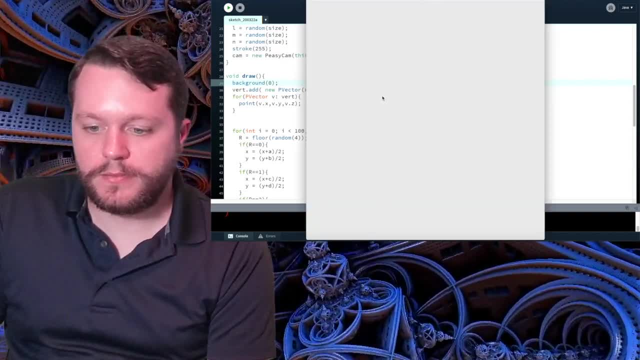 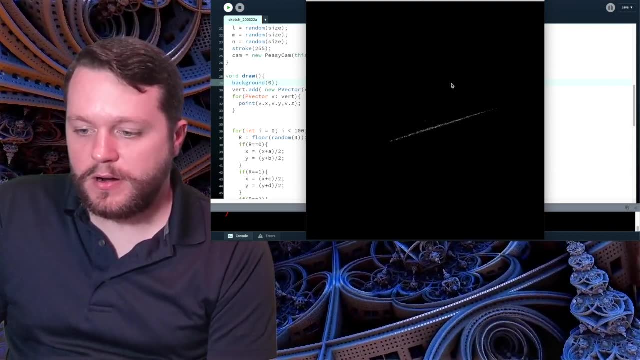 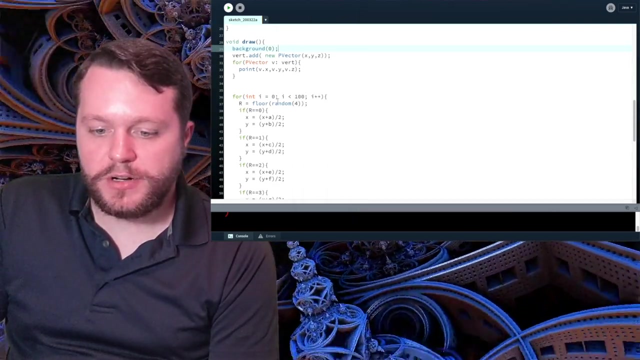 I just covered up, So I'll put that at the top. Oh, I just saw it There. it is Okay, cool. So here Now. the shape is still flat, So we need to make sure that each time we run this for loop here, a z direction is also being. 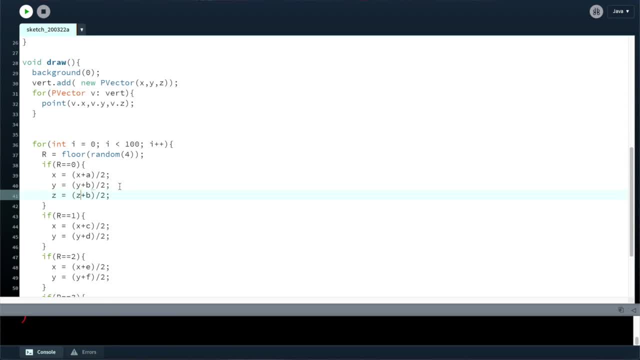 drawn, So z is equal to z plus We're going to change that to c, d, e and f. That is z Okay, d e, f, g, h, k, l, m and n. 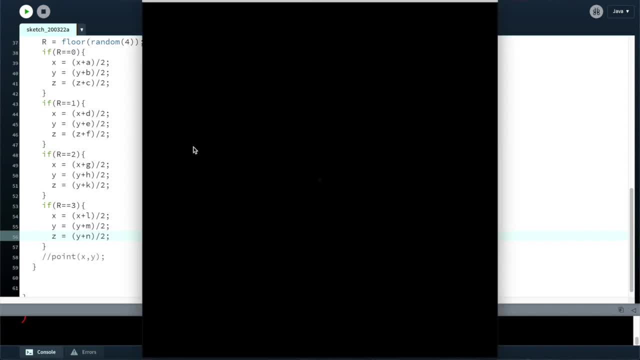 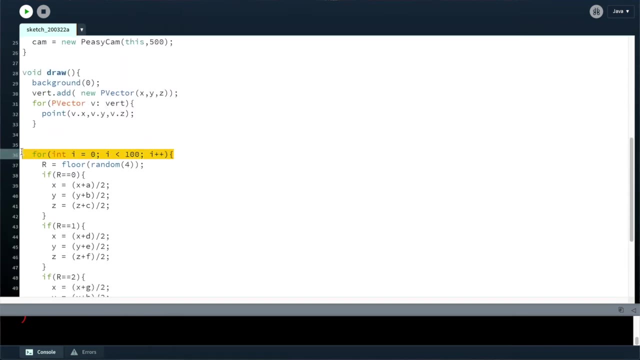 And I think with that: Oh you know what? That is pretty cool, But that's not exactly what we wanted. So I'm going to take all of this out of a for loop. Get rid of that. Don't need that anymore. 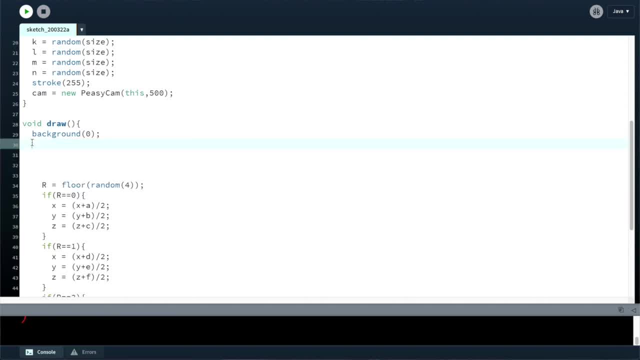 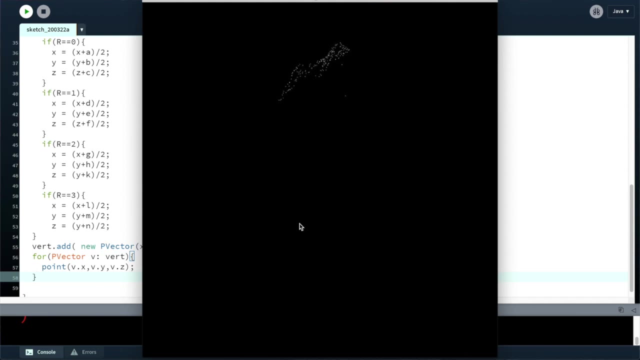 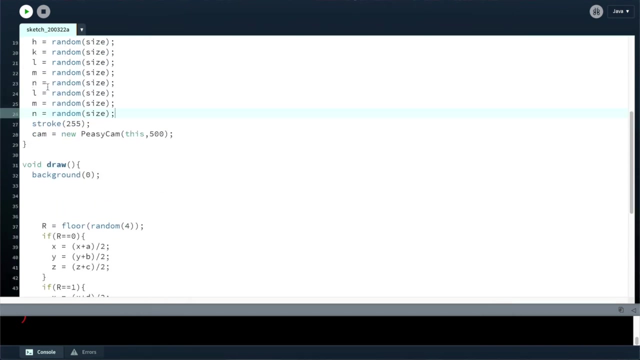 I'm going to move this stuff below here Now. that hasn't really changed anything. I'm just checking something to make sure we're good so far. So we still got that weird thing happening. So what is going on? So I'm going to make one more point. 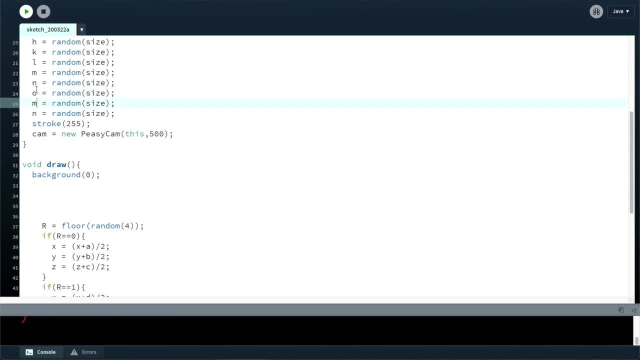 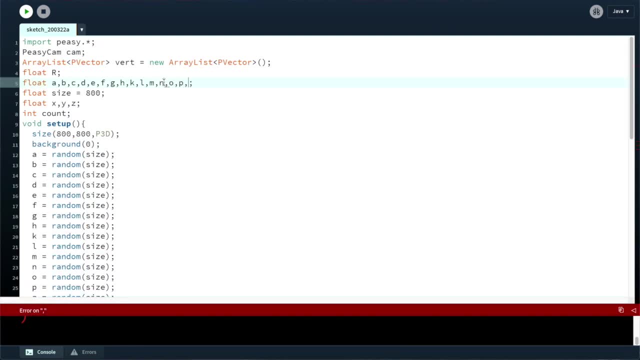 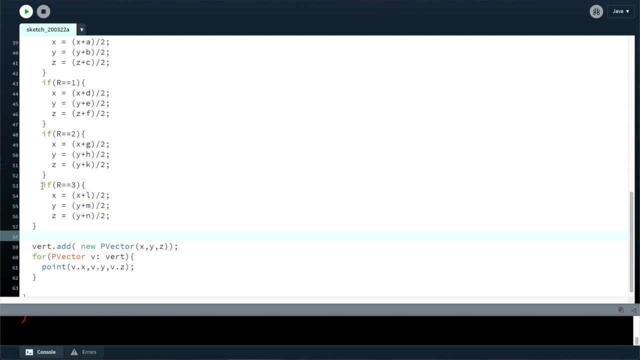 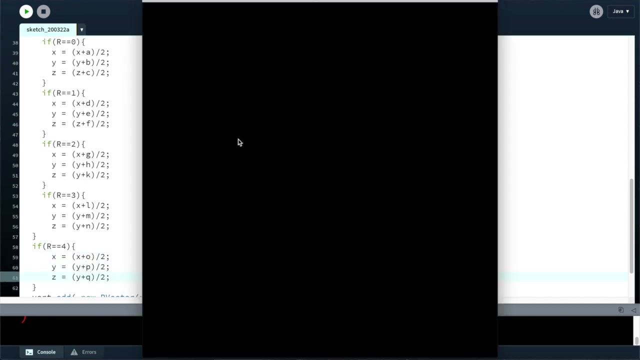 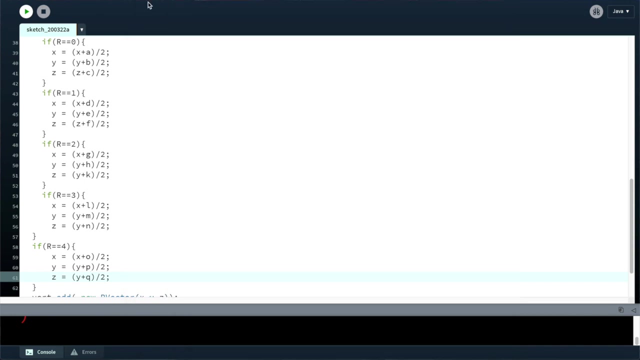 O, P and Q. O, P and Q, Just to make our fractal extra fancy. O, P and Q Cool. I guess I could translate it and scale it, But that's not going to do it. 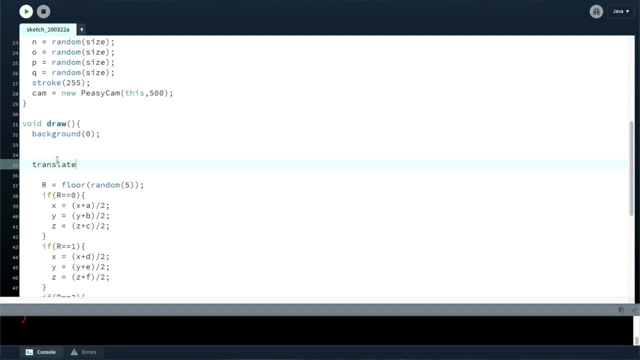 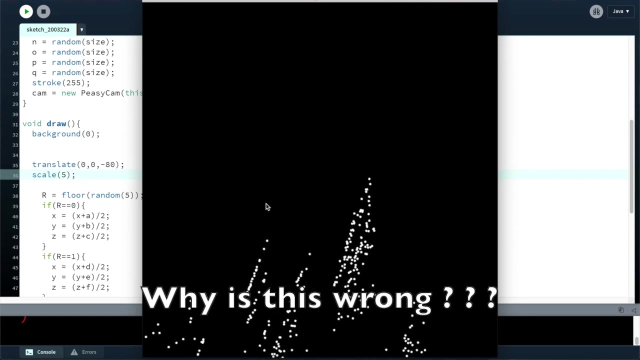 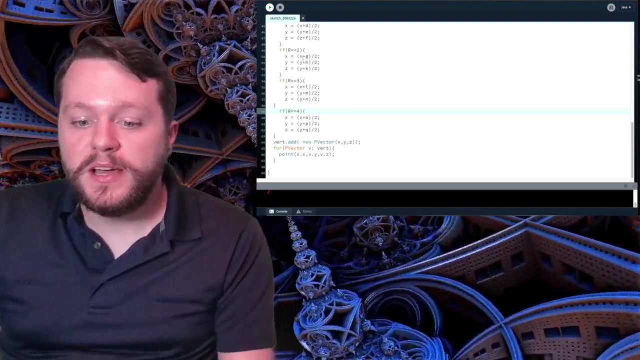 That's not going to change the shape of our fractal Three hours later. Okay, After taking like five minutes in debugging, I finally realized what was going wrong. So if you look right, here I am using Y for each of. 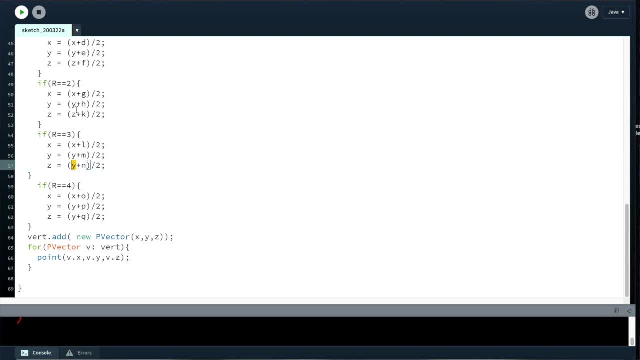 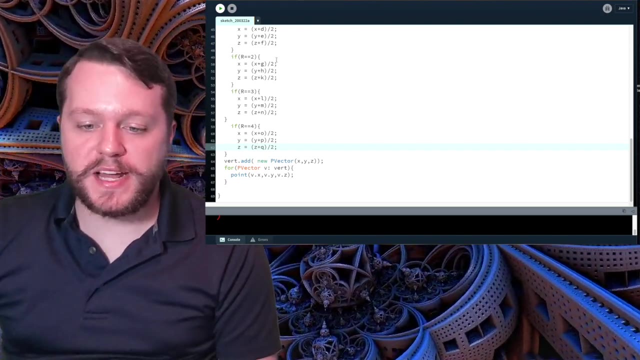 these, And that's not what we want. This is supposed to be Z, Z and Z. So that happens to me all the time. Guys, make sure you're checking what you're doing. Um, even if you are paying attention, you'll make simple errors, and sometimes it's a pain to go back and try to find, but that's. 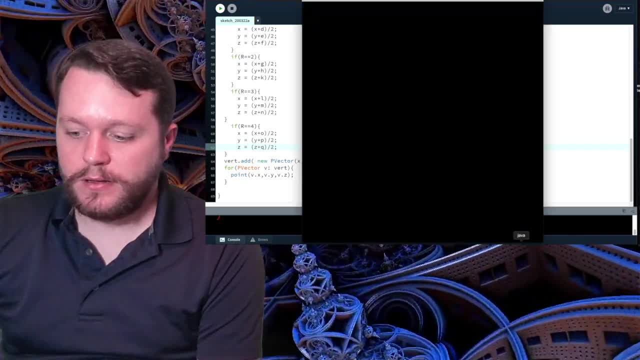 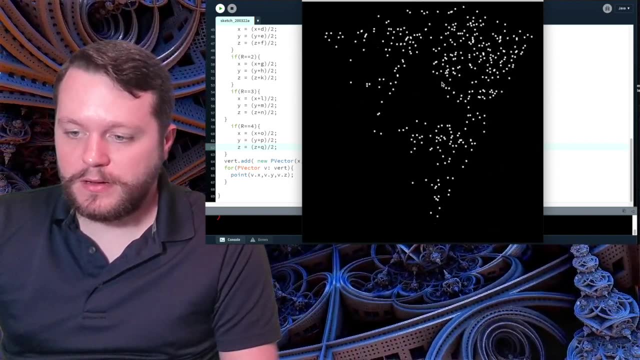 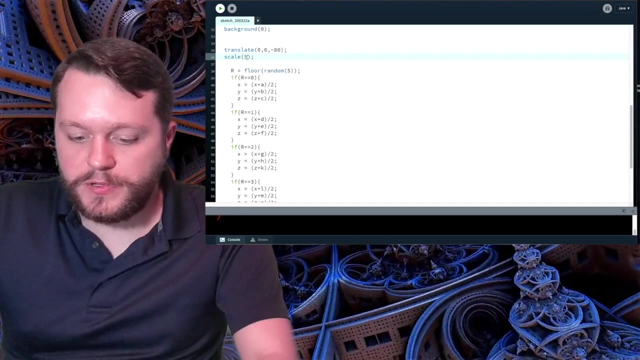 what was going on going wrong with this one. So if we run this now, we should have much more interesting fractal And yeah, that looks much better. Um, all right either way. Um, so it's working the way we want. So now we can do some touching up, So I'm going to actually back up. 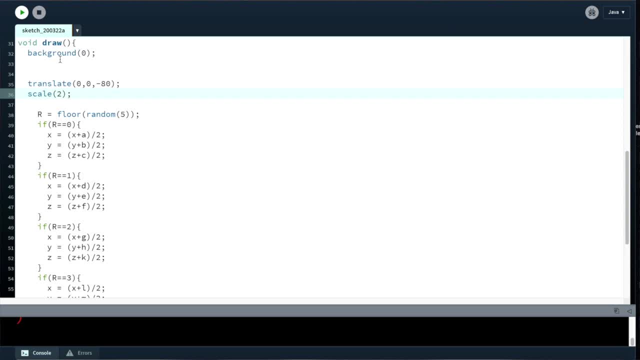 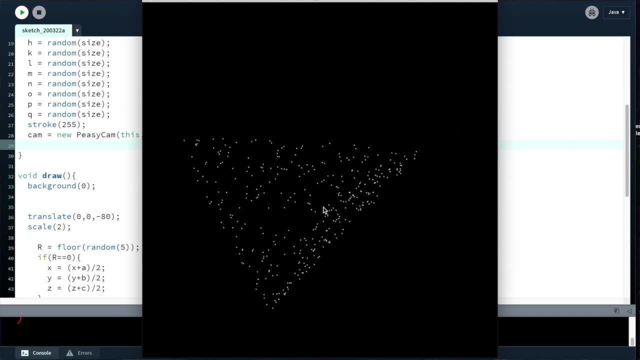 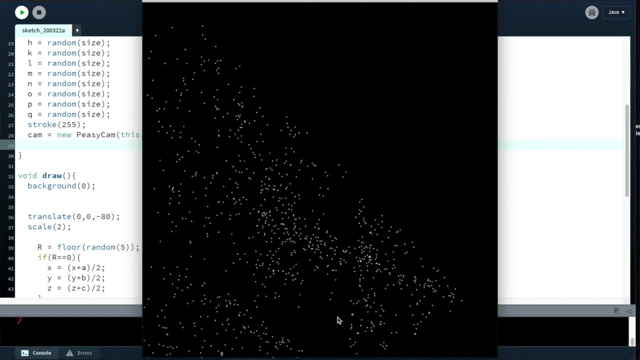 or make it smaller using the scale function here. Where'd we go? All right, cool Um. we've got a fractal generator that is in three dimensions. There we go. It's trying to back out so we could go in and explore it. That is super cool, Um. 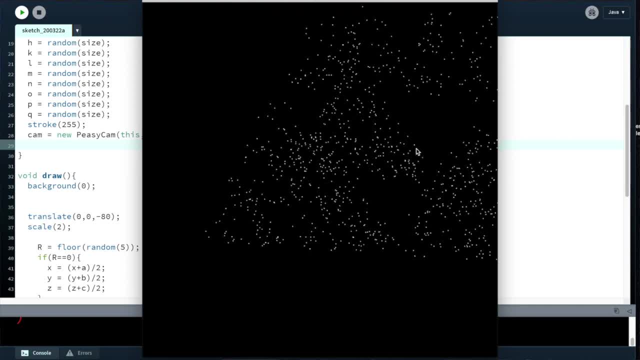 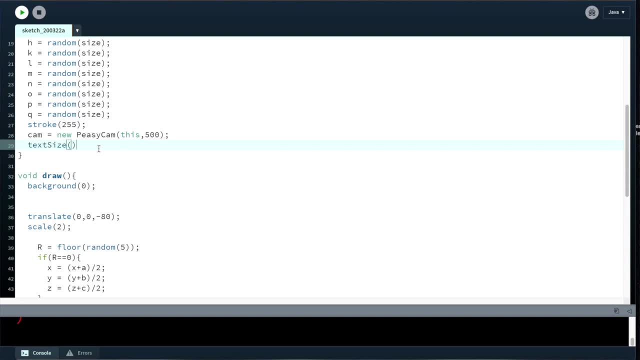 we could label each vertex. Why don't we do that? So I will say text size. Let's make it like 50 or something. Um, we'll draw text And actually I'm going to give it a fill of green. 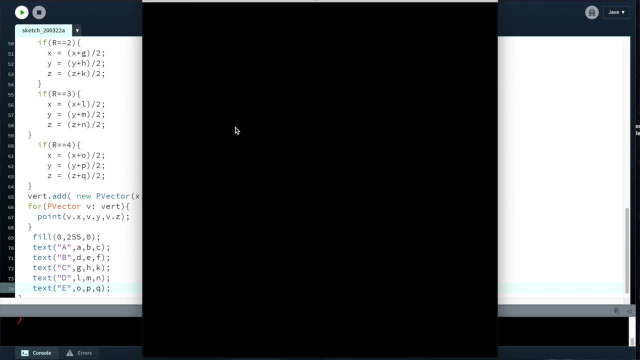 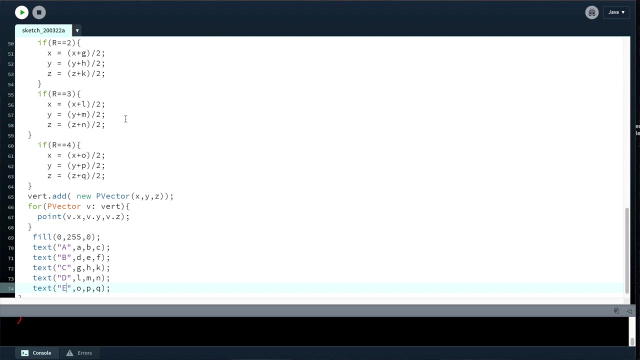 Okay, let's check that out. Nice, Nice, Oop zoomed out a little too much, Um. so yeah, now each vertex has been labeled and we can draw a line that goes from wherever the pixel in the last frame was to wherever the pixel in the current frame is. So I'm going to say 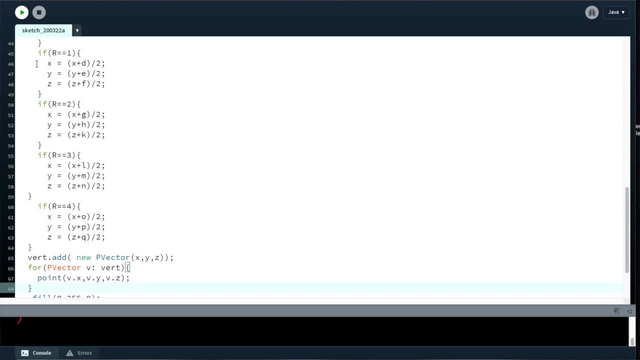 there's probably better ways to do this, but I'm going to actually run this algorithm right here twice. Between them I'm going to say um, And then we will draw. so it'll run that algorithm again and x, y and z will have new values And then we can draw a line which I want to have: the blue value I like. 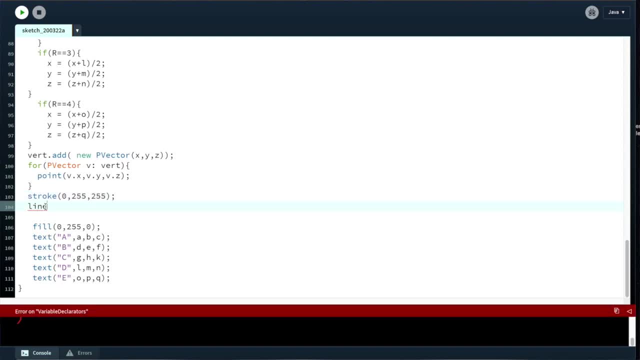 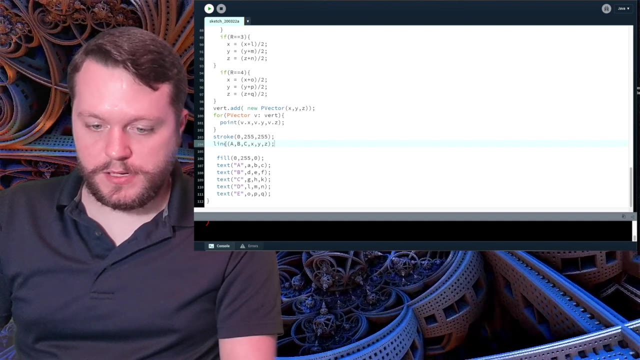 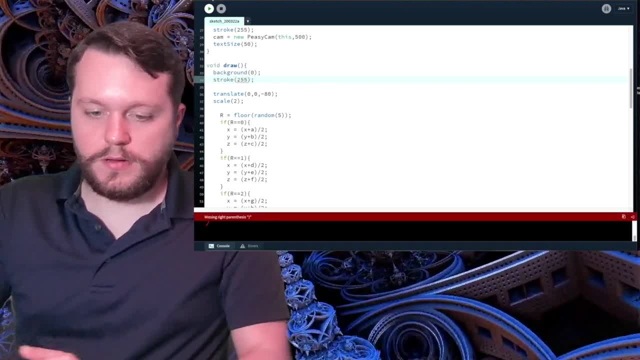 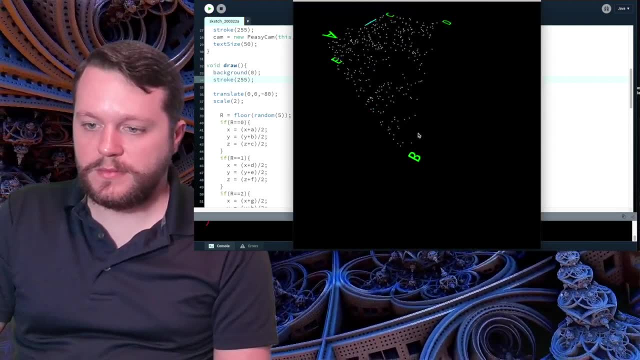 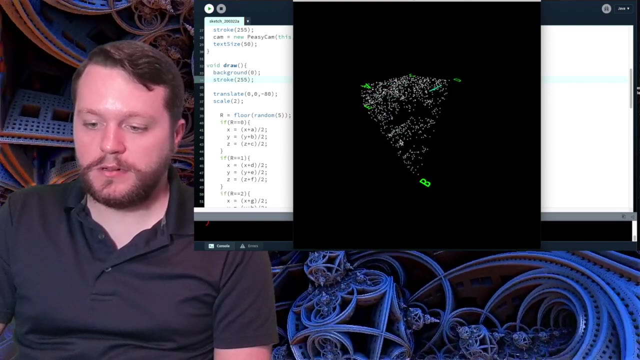 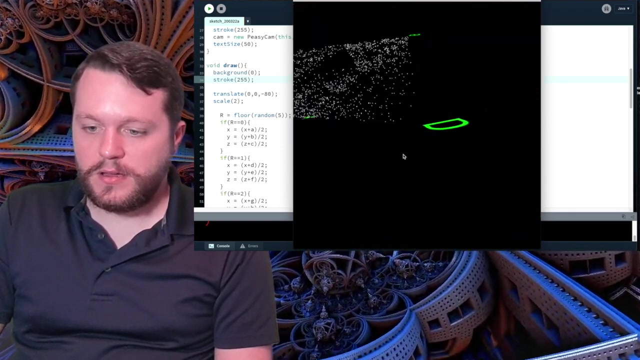 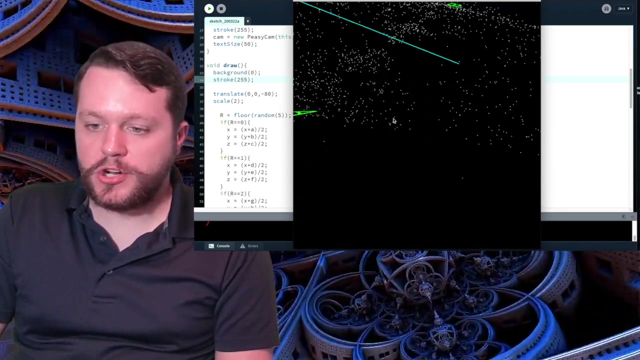 to white. All right, I think that will work. Yep, there we go. So it's drawing a line from wherever the last point was to where the current point is. That is super neat, And if you just let this run, this fractal will continue to get more and more sharp.